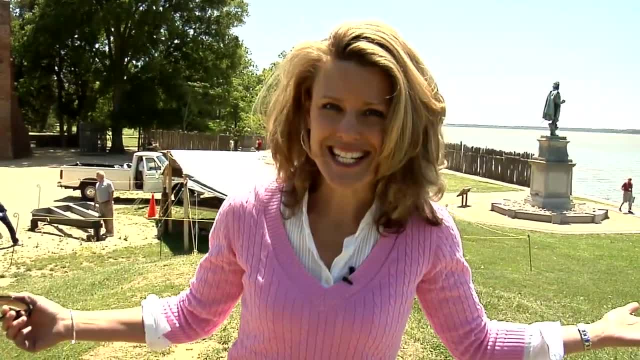 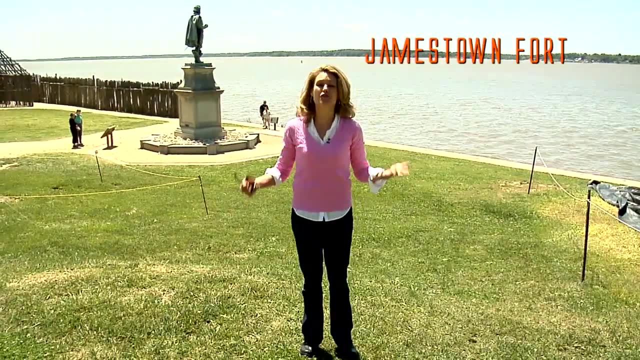 But first let's talk about where I'm standing. Get this: I'm standing inside a fort. That's right. and it's not just any fort. This is Jamestown Fort. It's the site of the first permanent English colony in what was then called the New World. 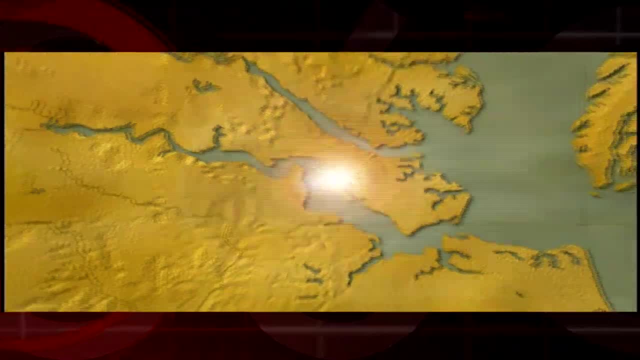 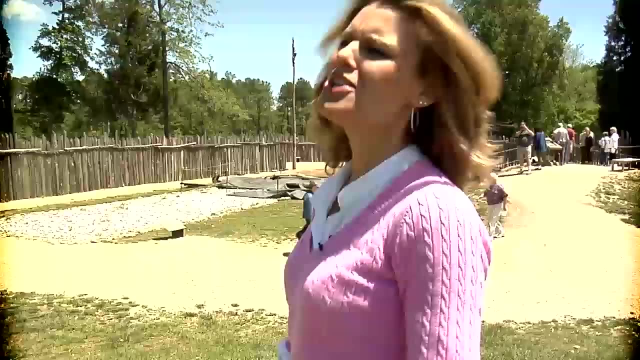 Today, of course, we know it as America. Now think about this From this starting point. people spread out all across the country and eventually populated the entire United States. So I guess we have to say that this landing spot is a pretty big deal in American history. 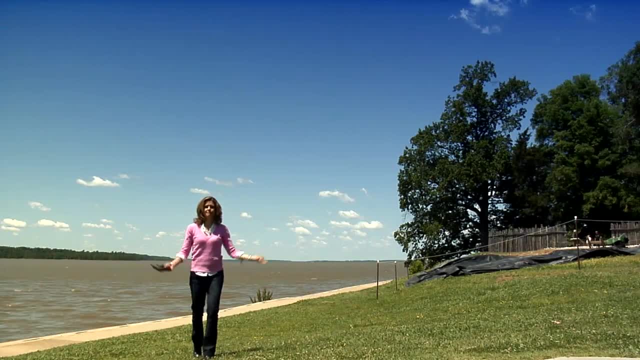 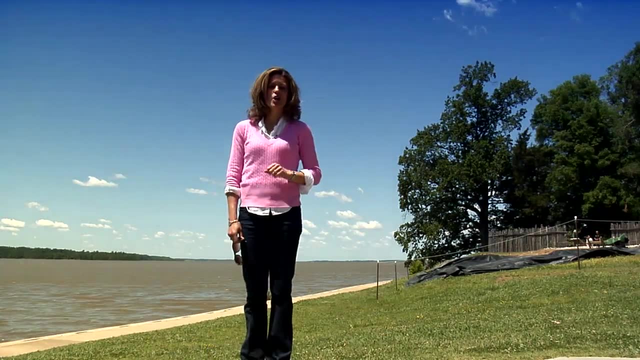 Over time, though, the original fort that the English settlers built fell into disrepair, Believe it or not, for many years it was lost to history. That all changed in 1996, when archaeologist Dr Bill Kelso rediscovered the original fort. 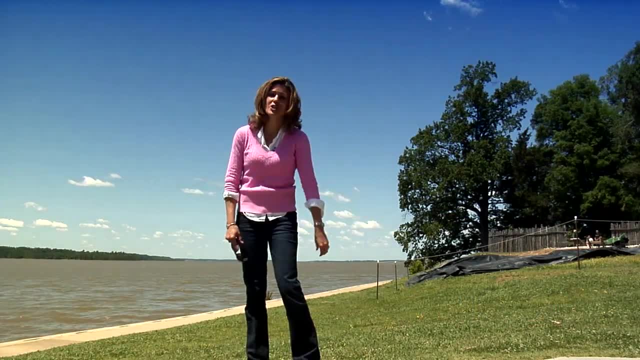 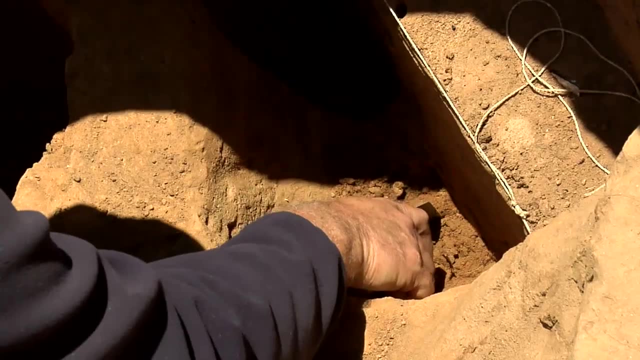 It began a whole new era of understanding What life was like for those first Jamestown settlers. For the first time they had proof, Using old writings, drawings and now a handy trowel for digging Dr Kelso and his team. 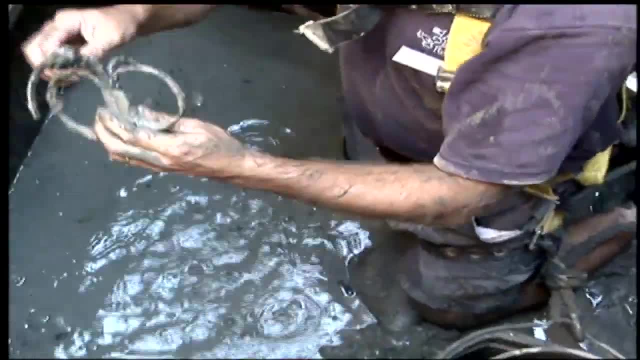 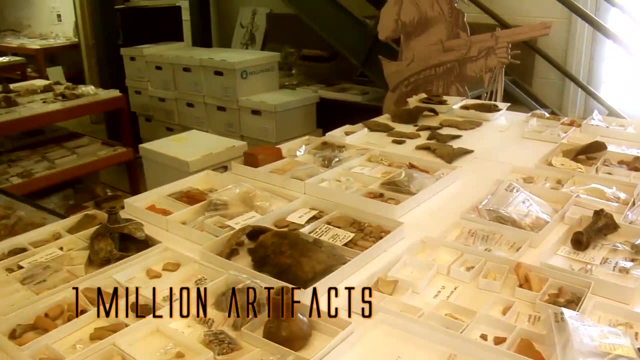 discovered where the old fort was and they began excavating the artifacts. To date, he and his team have found over one million artifacts from the original fort and they expect to find many more in the next few years. In a little while we'll catch up with Dr Kelso and dig a little deeper into the history. 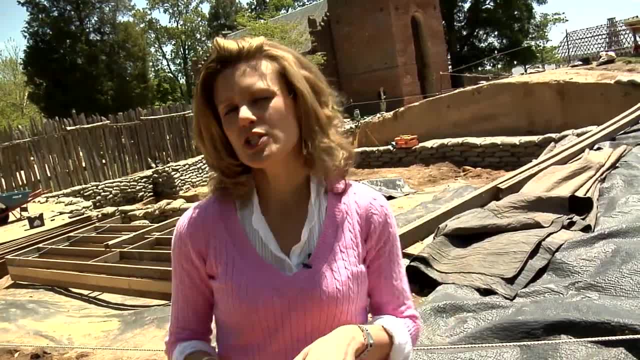 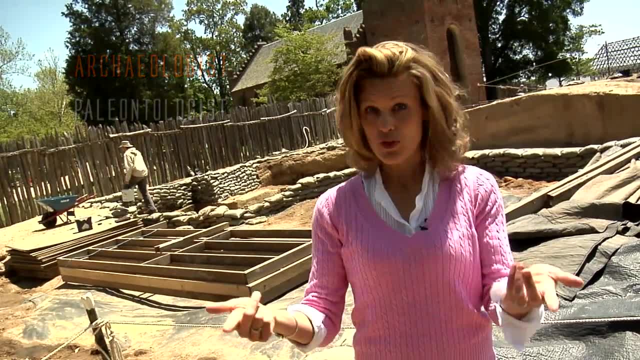 But first, do you know the difference between an archaeologist and a paleontologist? Well, let's see, They both dig in the ground looking for things from the past, right? Well, it's the type of things they're looking for that make them different. 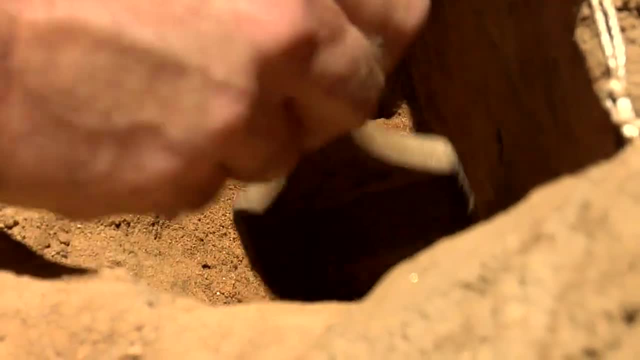 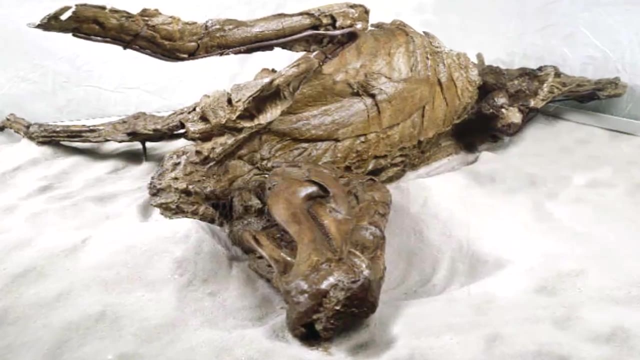 You see, archaeology is the science of understanding human cultures, while paleontology is the study of prehistoric life forms. So, basically, man-archaeologists spend their time trying to understand human cultures. But what's the difference? Well, archaeology is the science of understanding human cultures, while paleontology is the 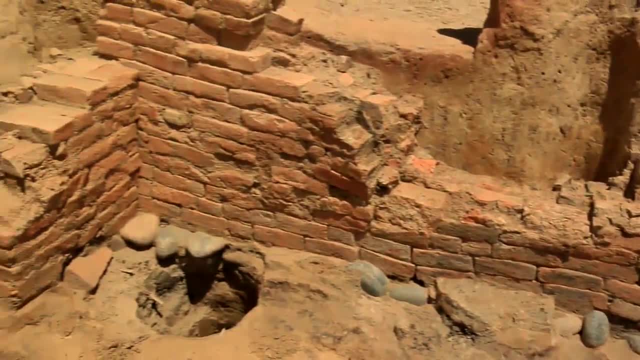 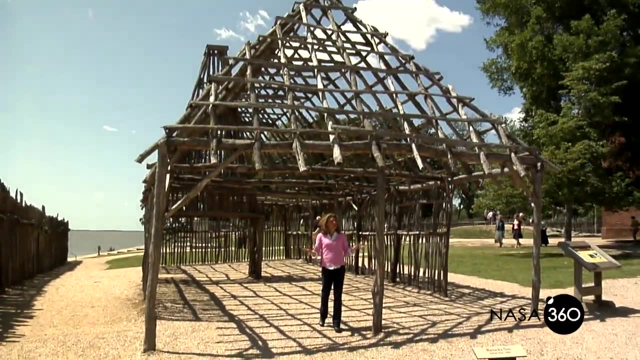 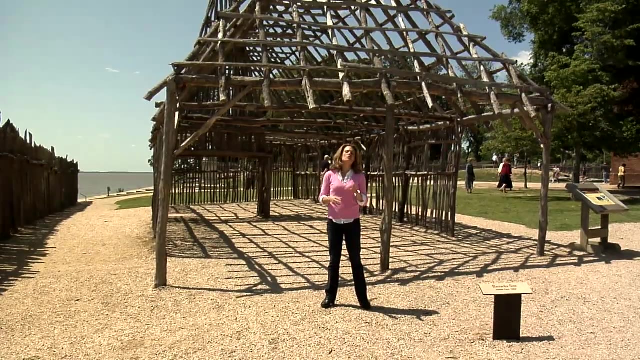 study of human history, while paleontologists generally look for fossils from before human history, Like dinosaur bones. Ha got it. Luckily for archaeologists and paleontologists, tons of help is now coming from NASA. How Well. one of the ways is through the use of remote sensing techniques. 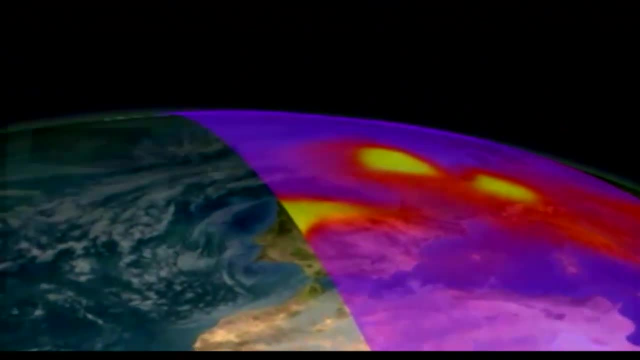 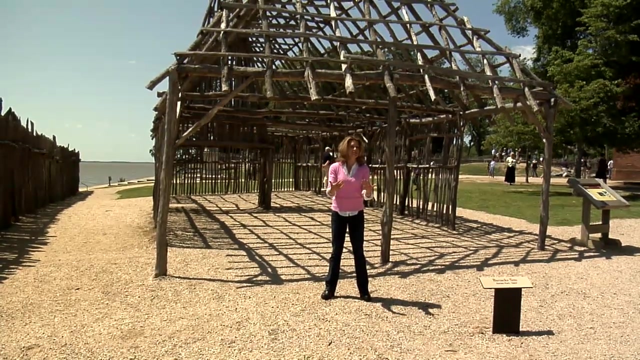 Remote sensing. Well, in the broadest sense, it's the use of a device to collect information without actually physically touching the objects. That's seemed like a long time. example of a remote sensing device we use every single day are eyes. Think about it. 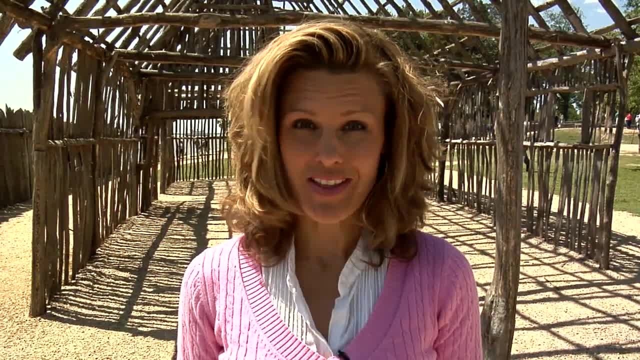 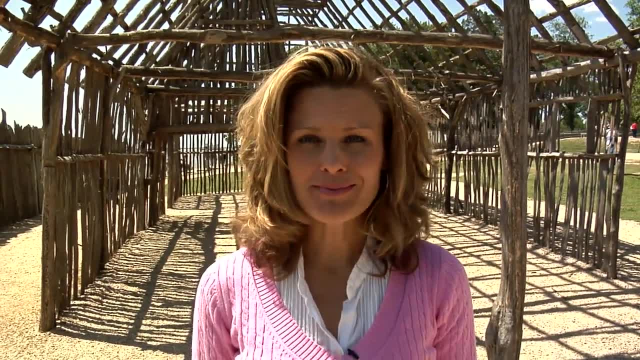 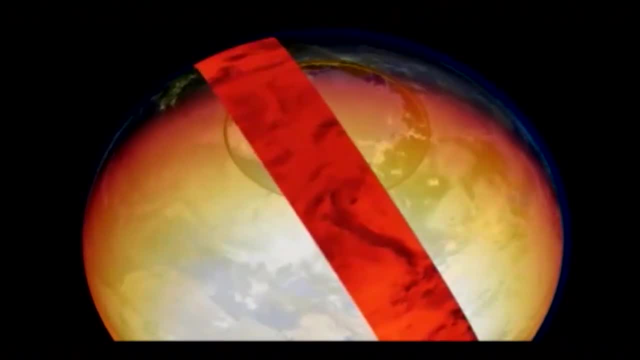 you can detect objects around you without physically touching them. You simply use your detectors or your eyes to see the object, gather information about it. you're using remote sensing. There are many forms of NASA sponsored remote sensing devices that are being used to help in archaeology and paleontology, Like, for example, there's something called 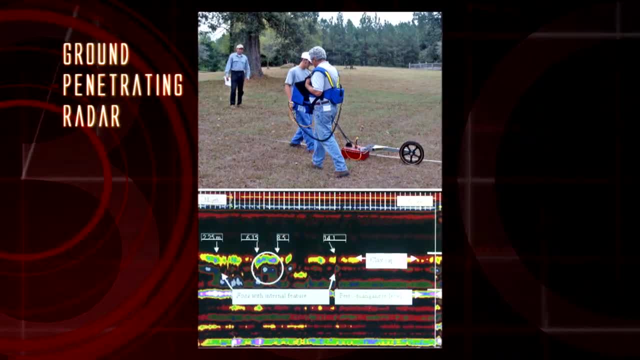 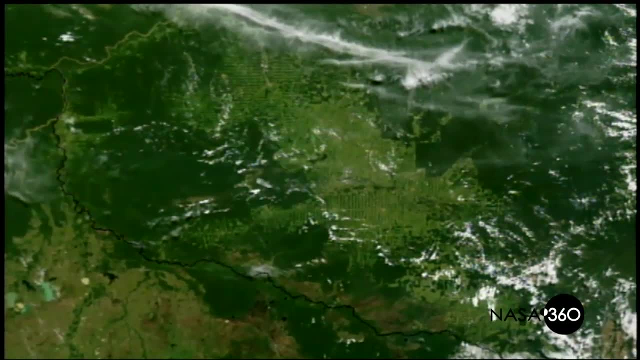 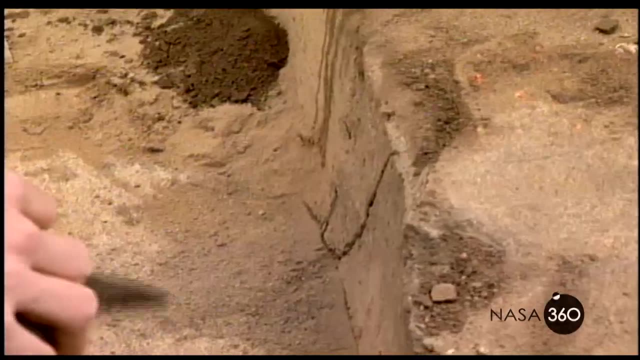 ground penetrating radar. This unique type of radar system can actually see objects in the ground without anyone having to dig them up. By using this, in combination with aerial photography and historical documents, NASA can help give researchers a much better indication of where to dig, what to preserve and what areas to avoid. Satellites are another type. 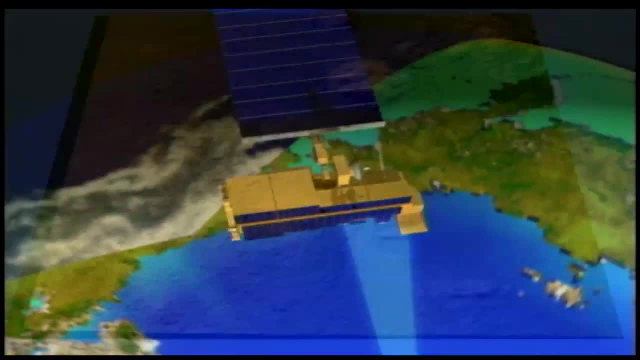 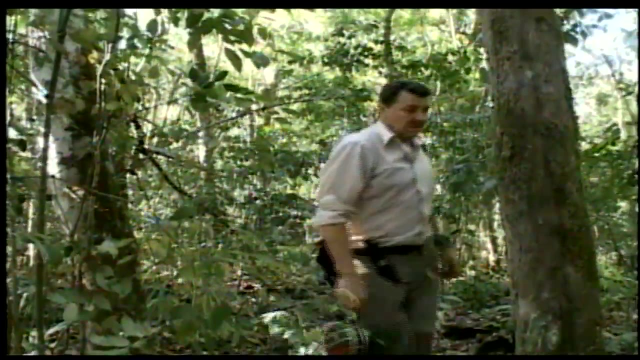 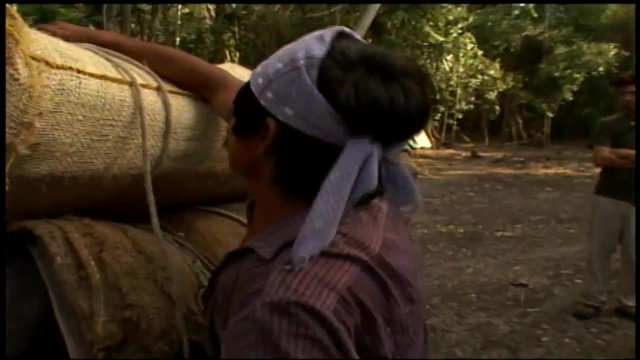 of remote sensing tool being used by NASA researchers to help archaeologists and paleontologists. In fact, NASA Archaeologist, Dr Tom Seaver, has been using satellite data to help us understand why the Mayan civilization in Guatemala Collapsed and how current populations may be able to prevent future disaster. 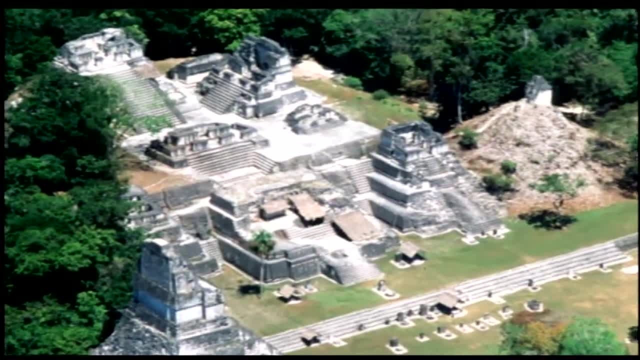 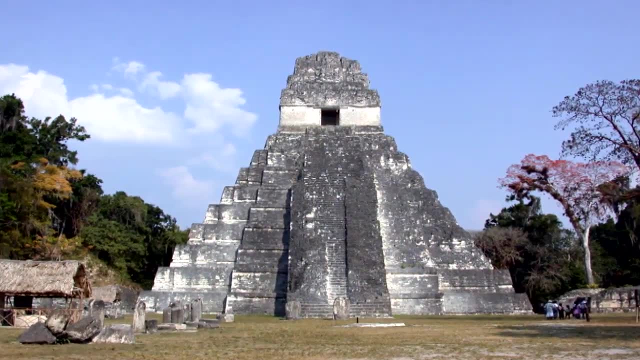 Let me try to break it down for you. between the 3rd and 9th century, the Mayan civilization in Central America Flourished, but after about the 9th century they collapsed, leaving Archaeologists few clues as to why this once mighty civilization disappeared. 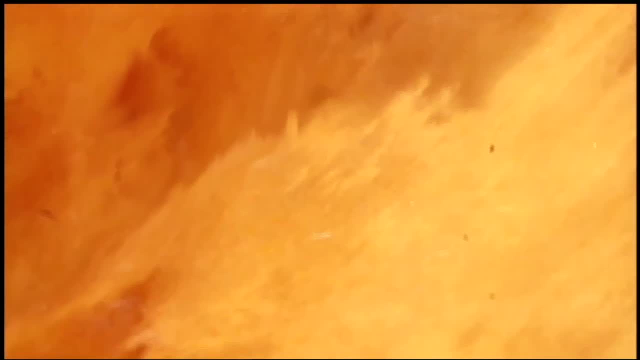 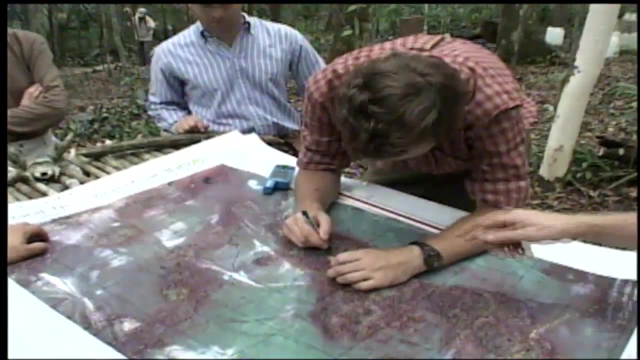 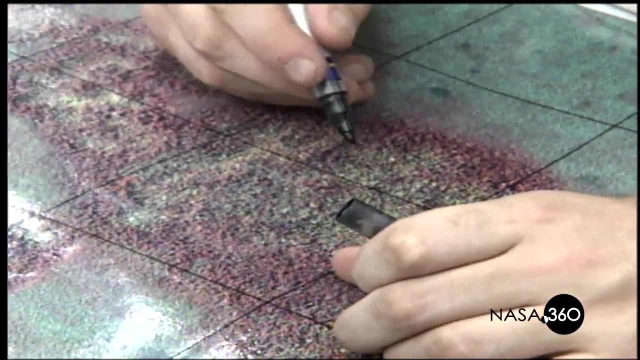 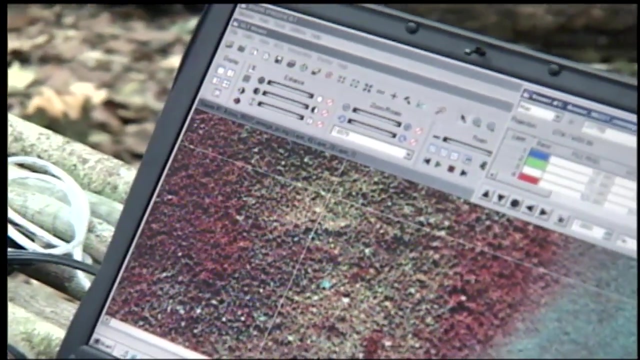 This is where NASA comes in. our remote sensing satellites can detect even small changes within the electromagnetic spectrum. so sand, cultivated soil, Vegetation and rocks each have distinctive spectral signatures which are easily distinguished from each other. so Archaeologists can use info from the remote sensing satellites to quickly target specific areas of interest, then send teams to that area. 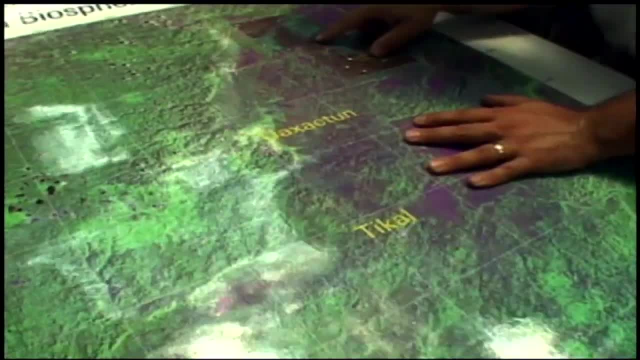 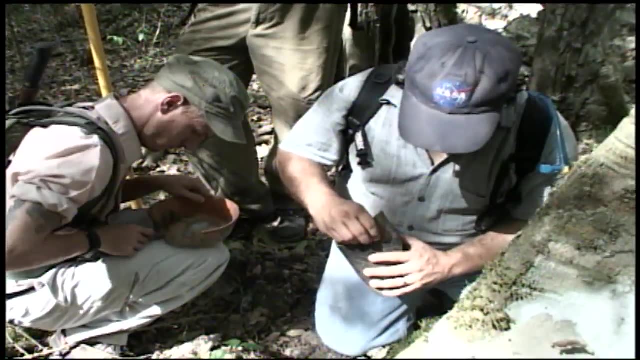 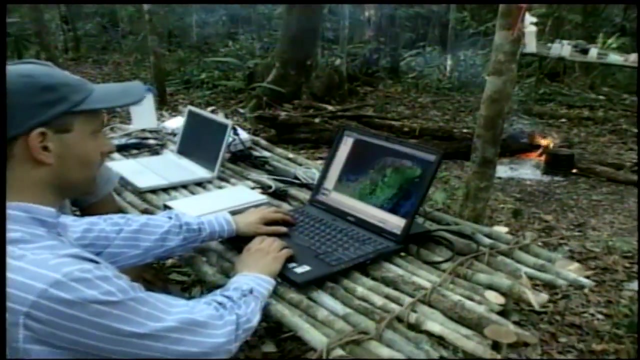 To validate the findings. dr Seaver and his team have already Found several previously undiscovered sites and feel confident that they know where others are, thanks to NASA's remote sensing satellites. That is how NASA is helping researchers find old ruins, But remote sensing satellites are also helping us understand why the Mayan civilization may have disappeared. 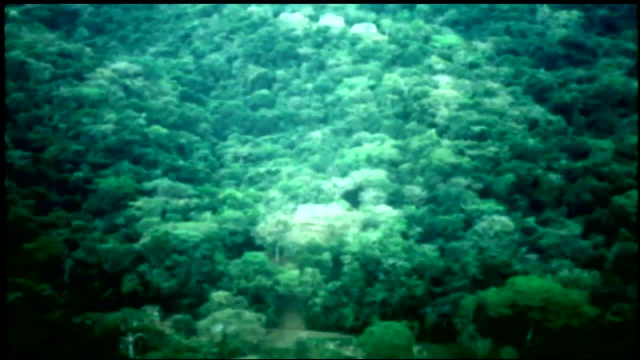 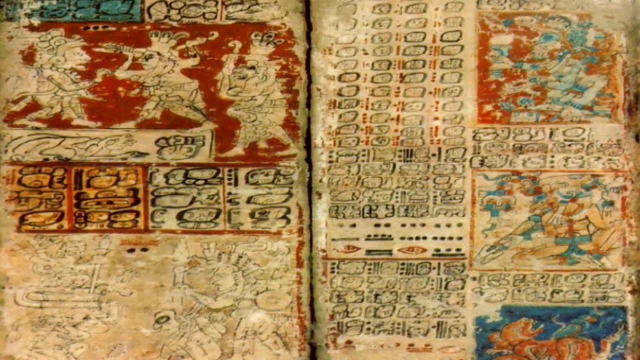 Today, the Patan rainforest in Guatemala is covered with trees. It's not heavily populated, but it was not like this during the peak of the Mayan civilization. in fact, during That time, this region had a population of about 2,000 people per square mile. 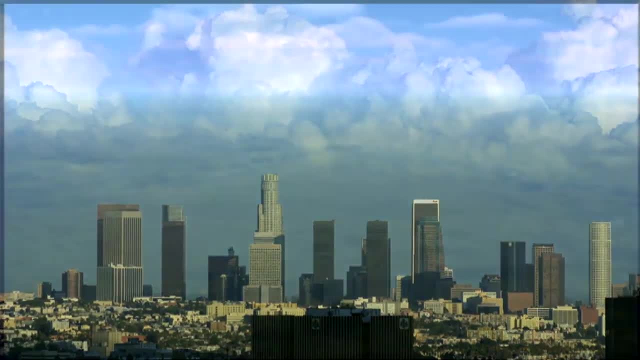 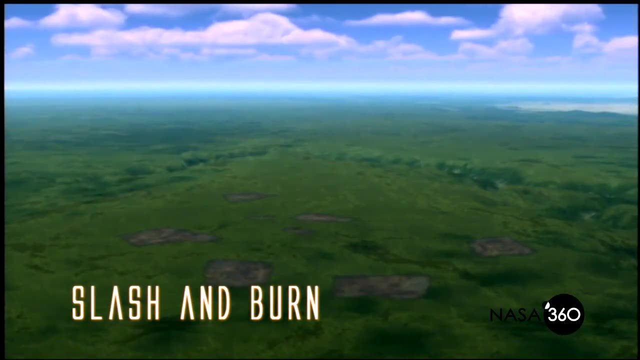 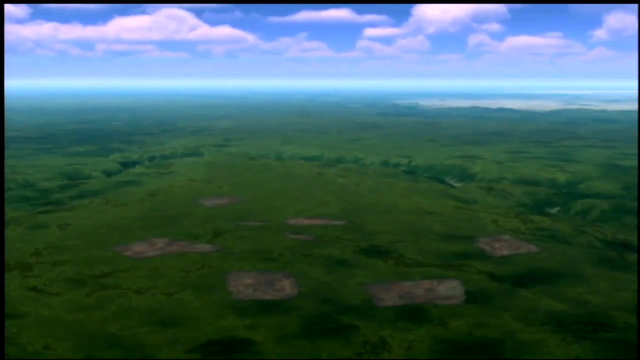 Which is about the same as current-day Los Angeles. with a population that large, the Mayas had to farm huge areas of land. to do this, They employed a technique called slash and burn, which eventually destroyed virtually every tree for hundreds of miles. Computer models show that as the trees disappeared, so did the rain, which caused temperatures to increase by five to six degrees. 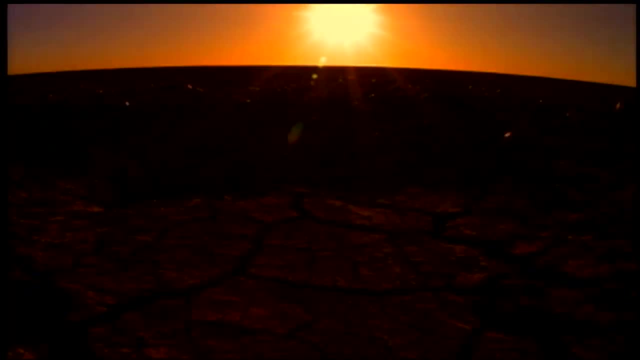 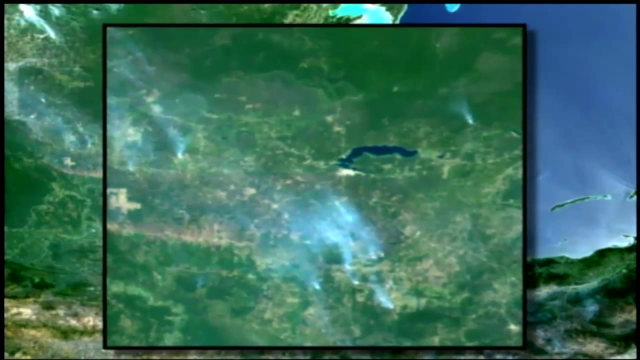 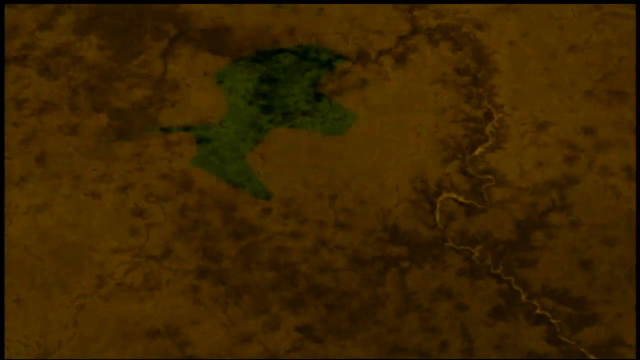 all of these shifts may have caused Malnutrition and disease, which, in turn, Contributed to its collapse. this information is especially important for us today, because slash and burn techniques are once again being used in the areas That were once Mayan strongholds. Understanding what happened to the Mayas may dissuade current generations of farmers from following the same destructive path. 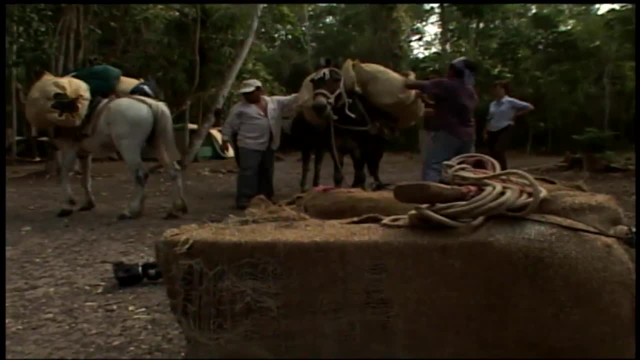 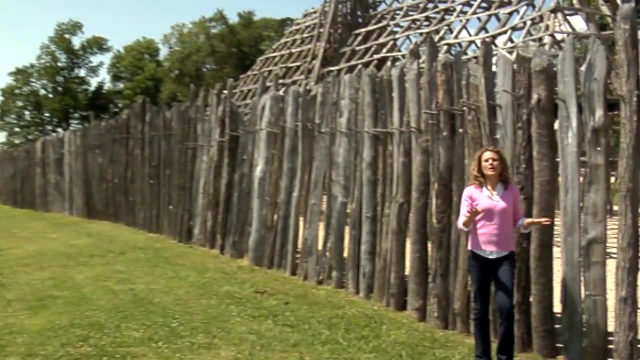 So, as you can see, NASA technology is being used for a lot more than just to help us in space. It's being used to help save lives back here on earth too. Hey, in a little bit We'll swing back out here to Jamestown to talk with Dr Kelso, but first 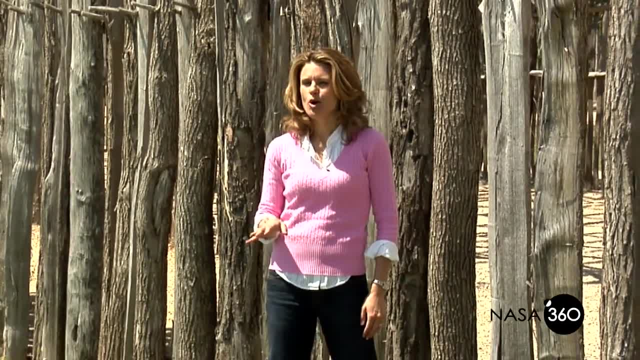 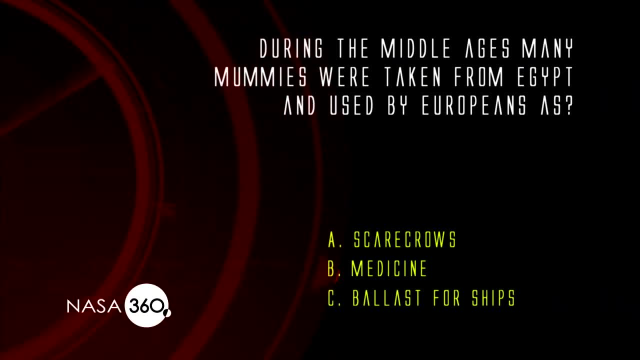 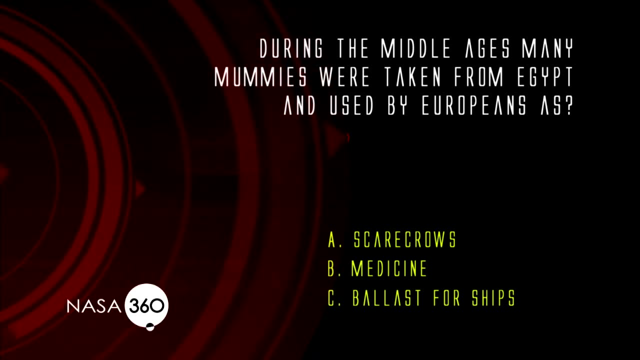 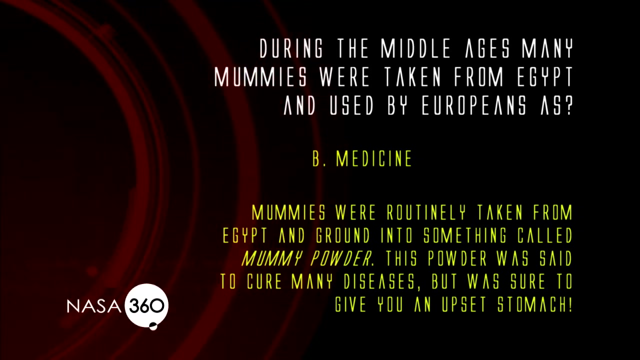 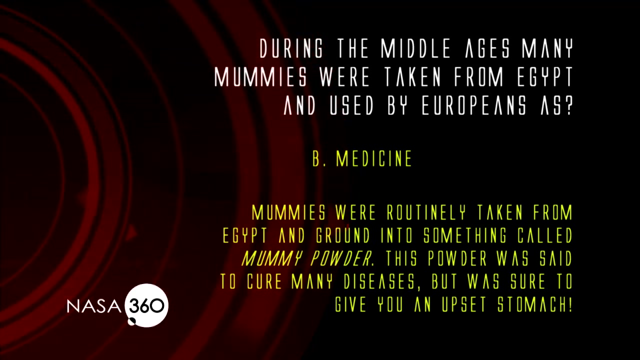 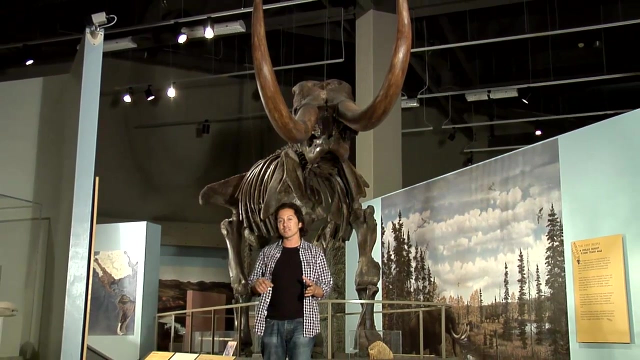 Let's head to North Dakota- Johnny Alonzo's there- to see what a mummified dinosaur and NASA have in common. hang on tight. You're watching NASA 360 Music Music. Hey, how's it going? Let me ask you something: Have you ever seen a real dinosaur? and then I'm not talking about one of those dinosaurs you might see in the movies, or 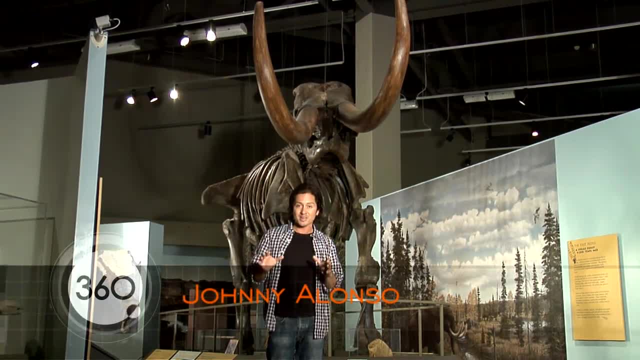 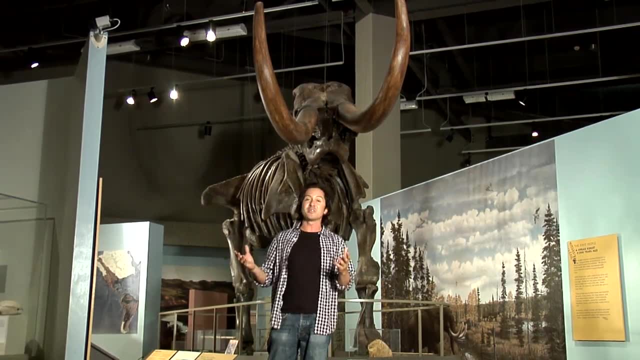 Even the skeletons in the museums. I'm talking about a real dinosaur with skin, muscle and bones. Yeah, it might be hard nowadays, considering the fact that dinosaurs live what hundreds of millions of years ago. but What if I told you that researchers found a dinosaur just like that? 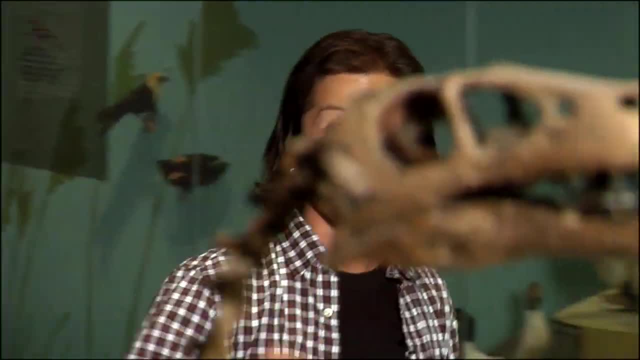 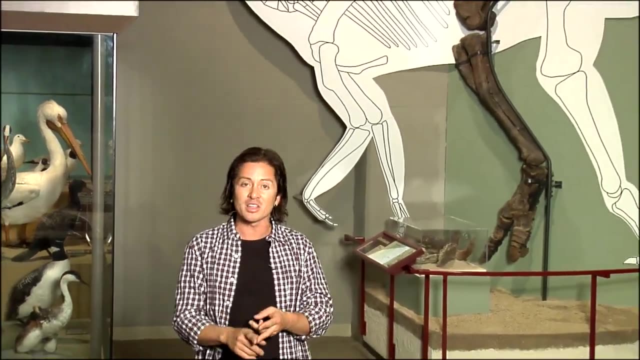 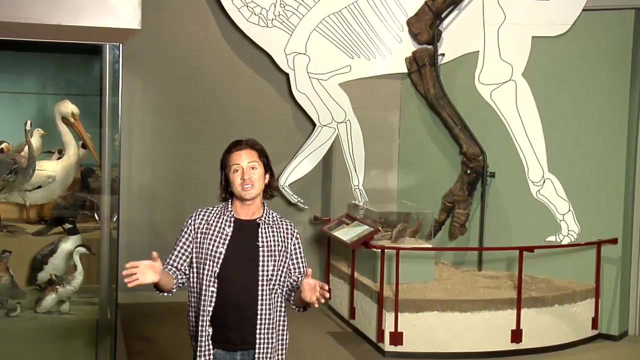 Would you believe it? well, if you said no, you better start believing, Because a few years ago, researchers found an actual mummified dinosaur that was still intact from the skin, the cartilage to muscle. a Mummified hadrosaur named Dakota is so unique in its discovery that it's changing what researchers thought they knew about dinosaurs. 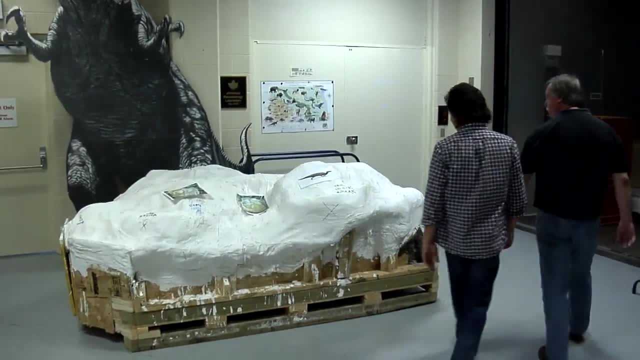 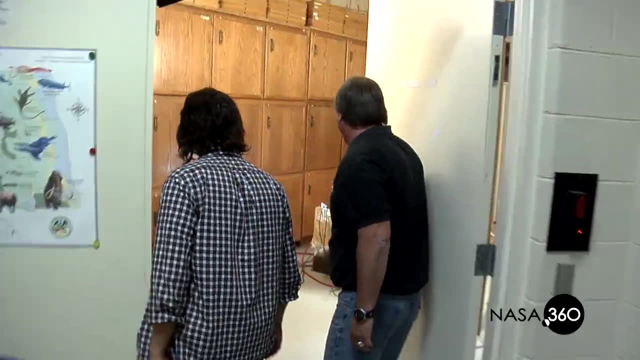 I rolled out the Bismarck, North Dakota to speak with my buddy, Dr John Hoganson, about this amazing discovery and to find out how NASA is helping unearth more clues. Wow, are you kidding me? Yeah, this is the. this is so cool. This is the tail section of the. 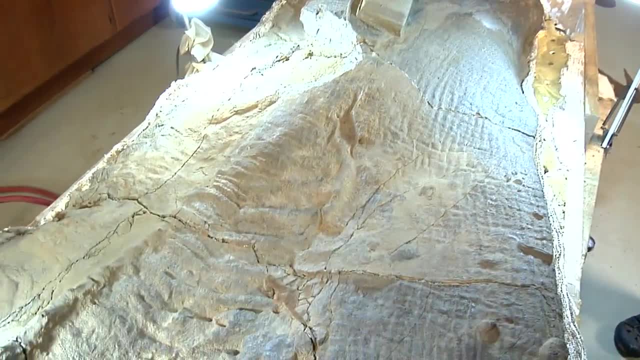 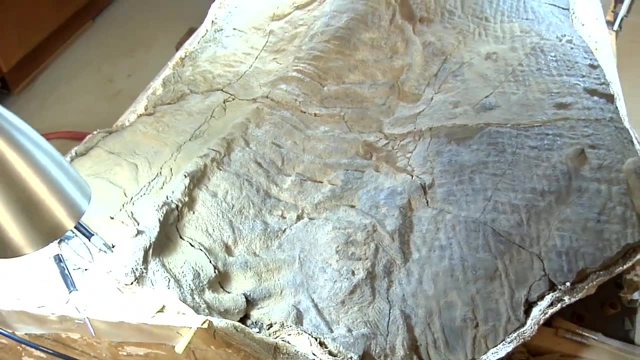 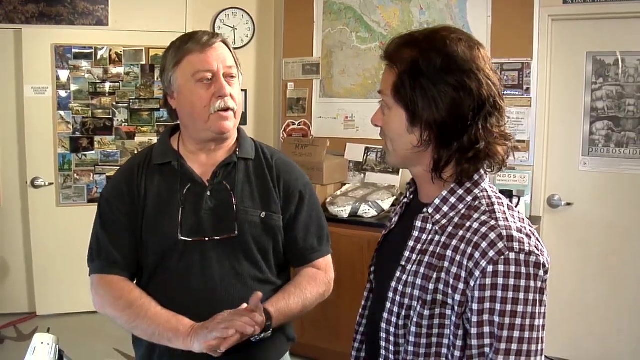 duckbill dinosaur called Dakota and it's being prepared here at the North Dakota Geological Survey Preparation Laboratory here at the Heritage Center in Bismarck. This is something else. Wow, It's a duck. How was this dinosaur found? Well, this fossil was found in 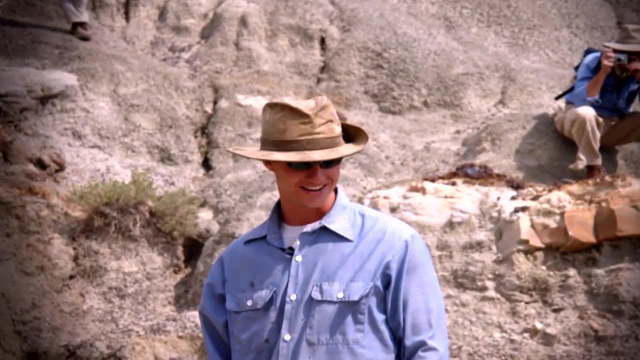 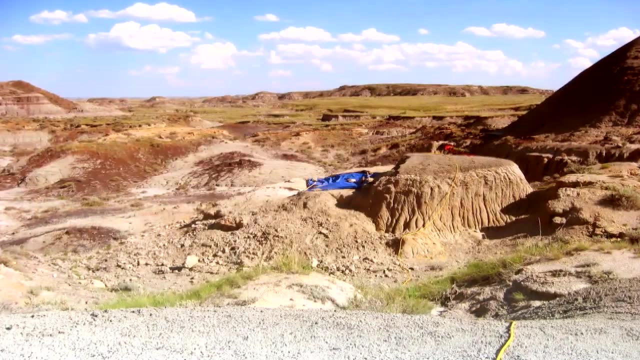 1999 by Tyler Leeson down in Marmoth, North Dakota, which is in the southwest corner of the state. He was only a sophomore in high school at the time But was out exploring for fossils, actually on his uncle's property down in the Badlands. Now This is a hadrosaur called. 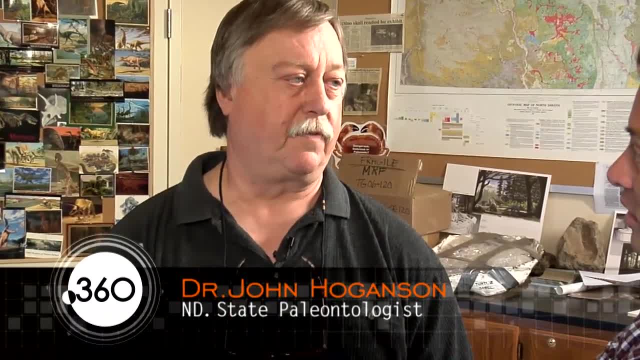 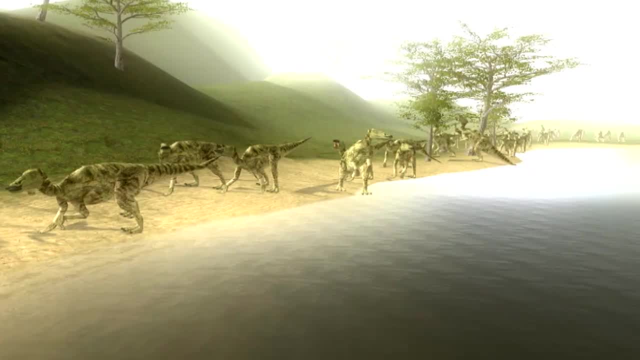 Edmontosaurus- that's a scientific name for this particular species of dinosaur Hadrosaurs- were duckbill dinosaurs. They- there were a group of dinosaurs that were referred to as duckbill dinosaurs because they're They have these little canisters, and then their snouts were compressed. 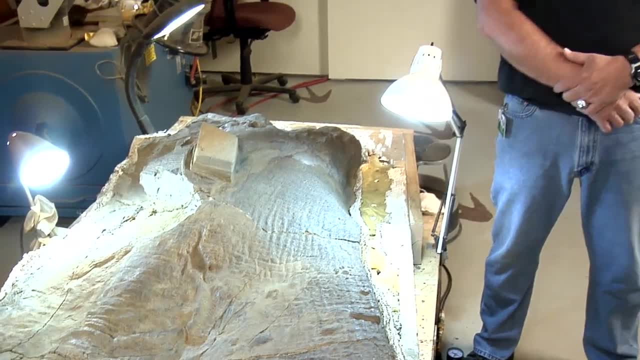 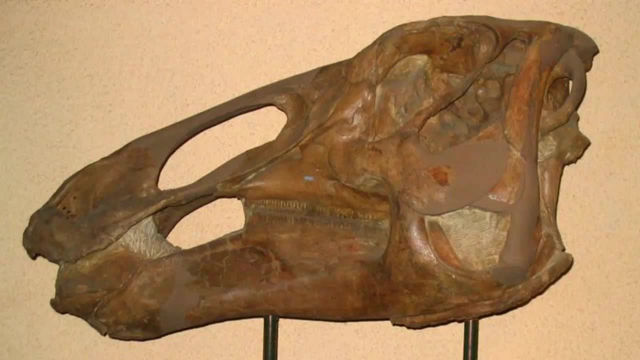 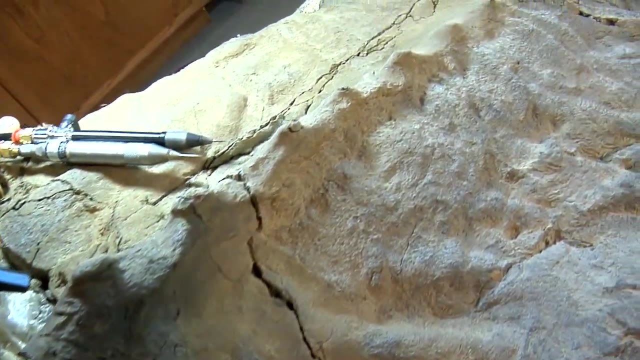 And it's very similar to a modern duck. So what is so unique about this fossil? Well, you know, generally paleontologists, when we're out exploring for fossils, will only find Individual bones or fragments of jaws or things like that. this particular dinosaur called Dakota is. 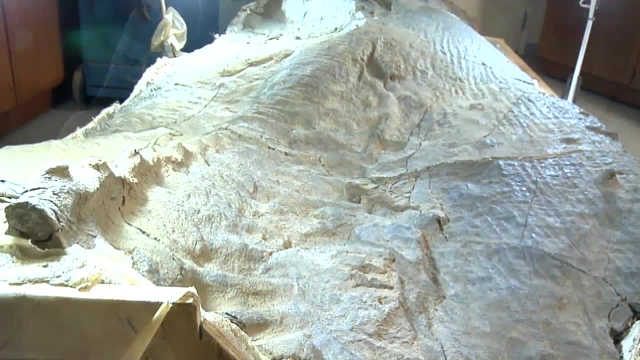 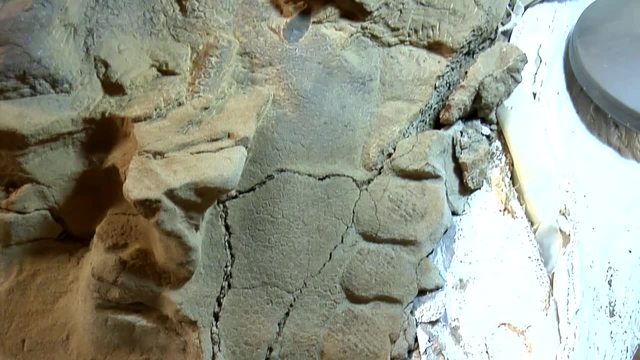 Not only a complete skeleton, but it's very unique because The skin is actually preserved on this animal, So wrapped in the skin that it was enclosed in. This is called a mummified dinosaur, but it's not a mummy in the sense of what we generally 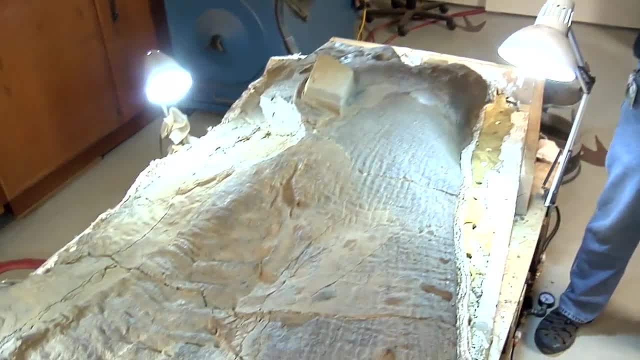 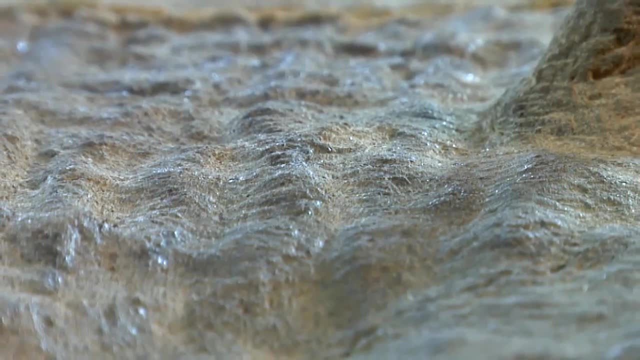 think about like an Egyptian mummy that has been embalmed for preservation. The skin on this animal is actually preserved because it's been replaced by a mineral called siderite, which is an iron carbonate kind of mineral, which is very hard and has preserved. 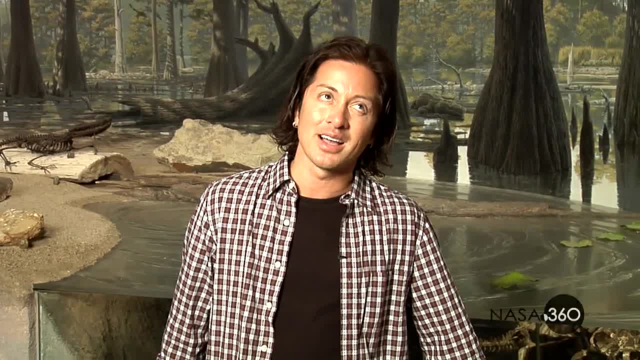 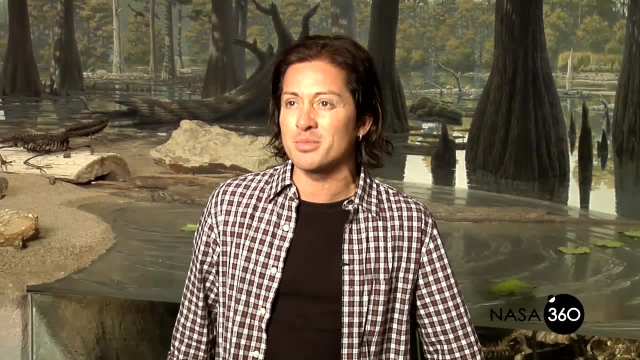 the skin, All right. so how did NASA get involved with this dinosaur discovery? Well, researchers needed a way to scan through all the layers of rock to see all the dinosaur, and since this thing weighs about 10 tons, they needed a really, really big scanner. 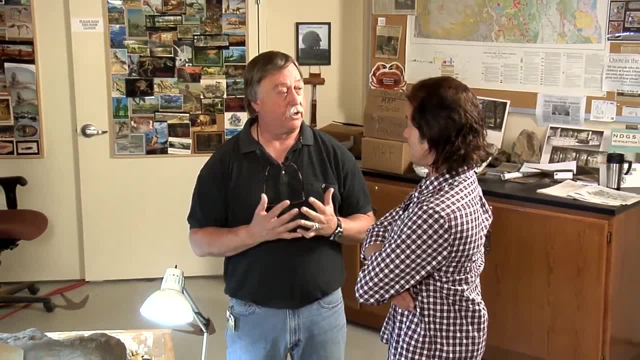 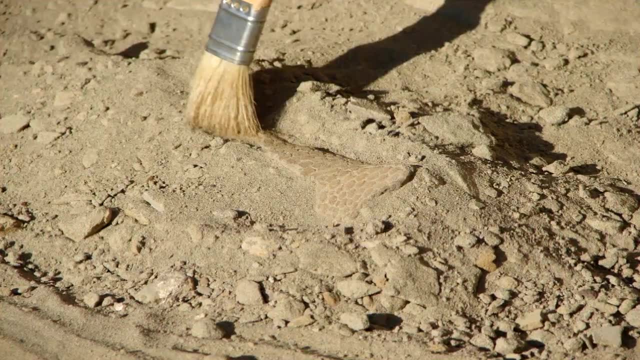 Well, you know, when we usually find these fossils in the field, we generally just find the bones, the skeletons, and it was determined early on during the excavation process that this particular dinosaur was covered in skin. So it was decided to take these. 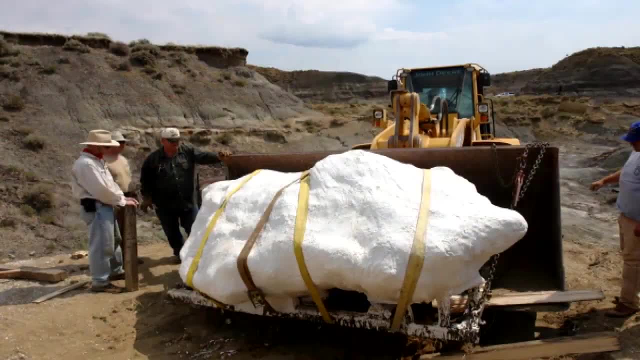 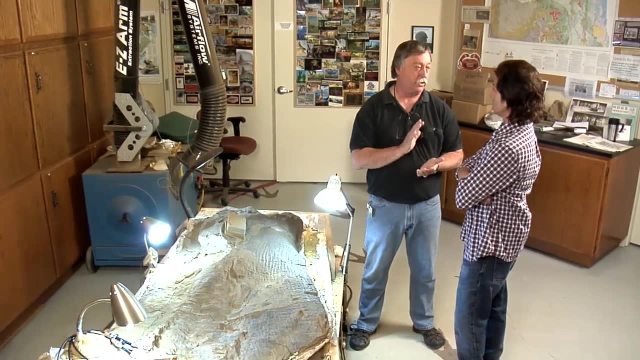 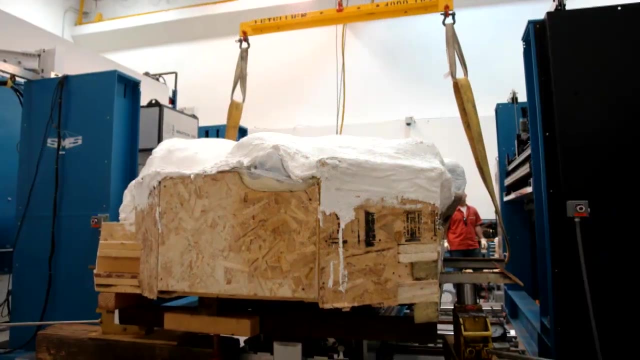 These skeleton blocks out, still entombed in the rock. so big blocks of rocks were removed And at that point it was decided that the best technology to use to determine the position of the bones in the rock and the completeness of the skeleton was to use CAT scan technologies. 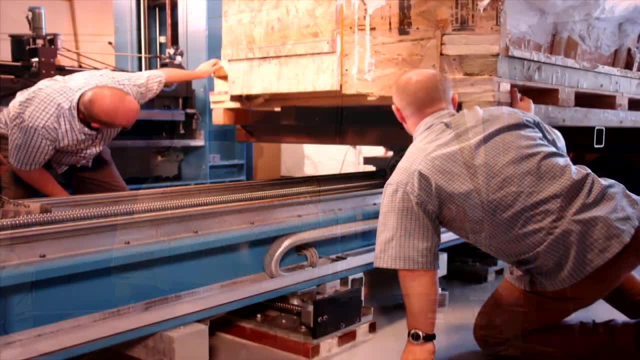 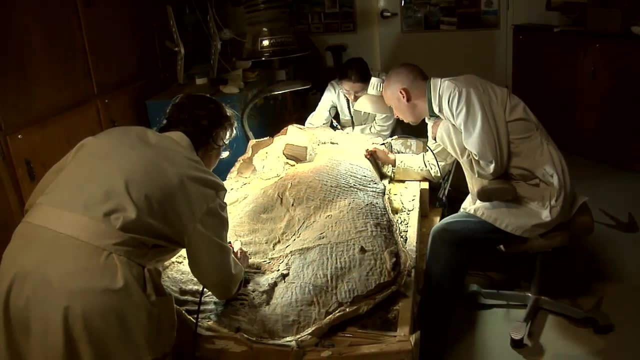 and that's where NASA was asked if they could help with this, And it's been a very good approach because, with this tail block that we're working on right now, We, through the CAT scan technology, are able to know where the bones are before we actually 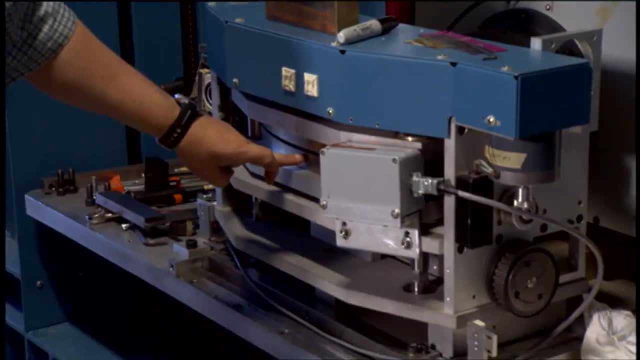 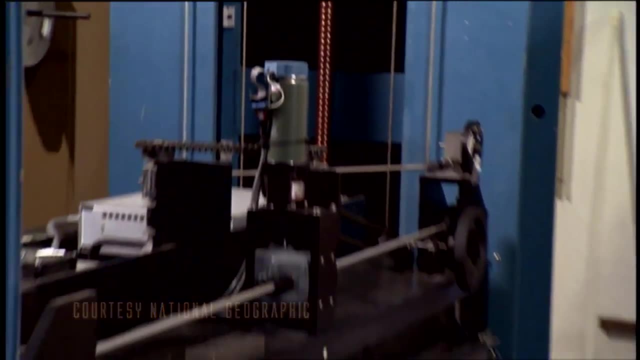 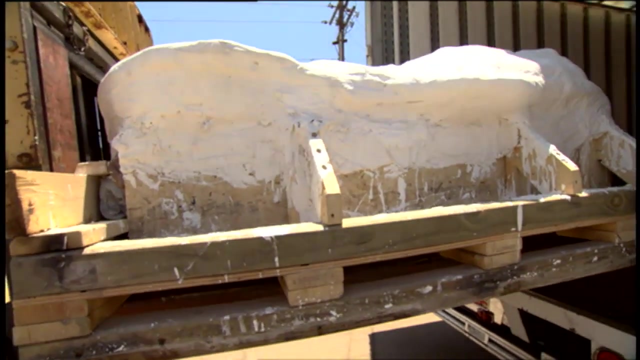 start digging through the rock matrix. Luckily for these guys, NASA operates the largest CT scanner in the world. Located at a Boeing facility in Canoga Park, California, this scanner's first priority is to inspect large space shuttle parts. Well, the task for Dakota was not all that different, so they loaded Dakota on a truck. 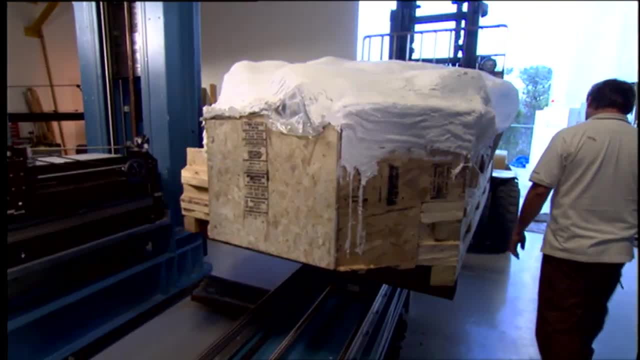 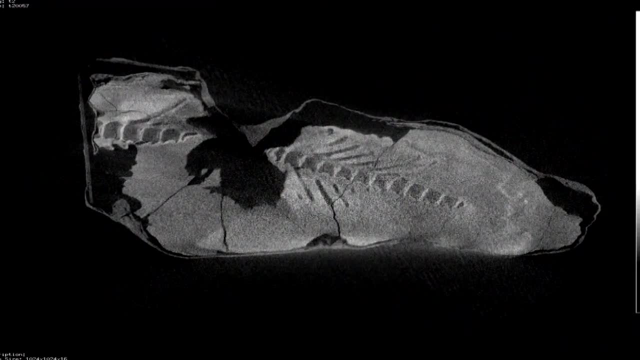 and shipped it off to California. When it arrived, the scanner was able to penetrate the dense iron carbonate that surrounded the dinosaur's tail section, and right away. researchers saw bones, tissue and cartilage. Well, since I've been a paleontologist, which has been a few years, there's been a lot of. 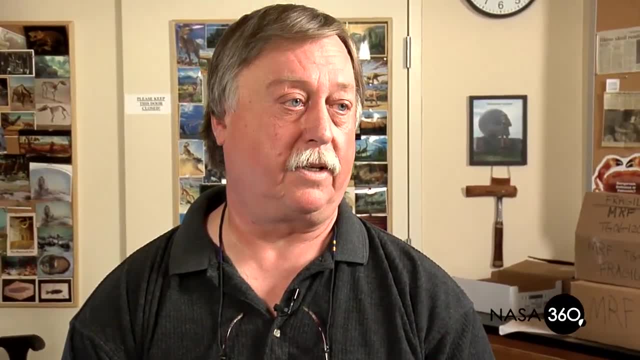 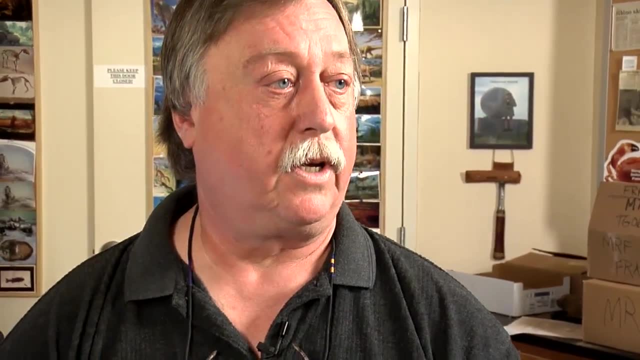 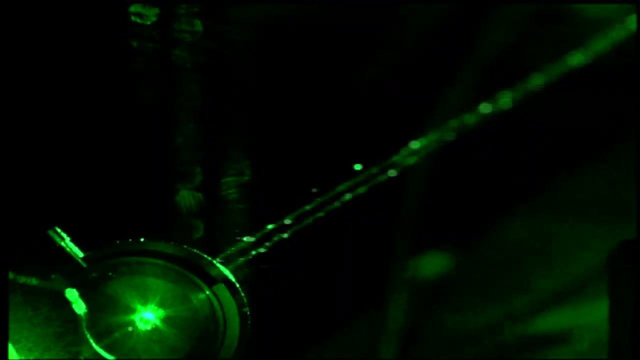 technological changes and advancements that have really helped the science. In addition to the CAT scan technology that we've been talking about here, there's a lot of remote sensing type of technologies that are available to us now: global position systems, mapping, LIDAR, kinds of laser mapping. 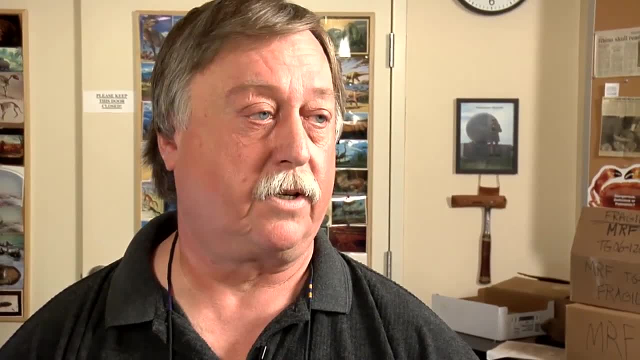 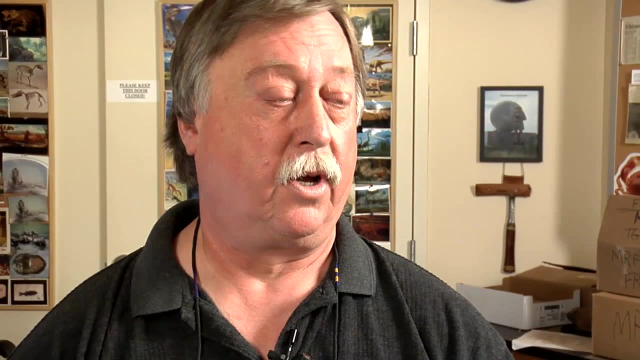 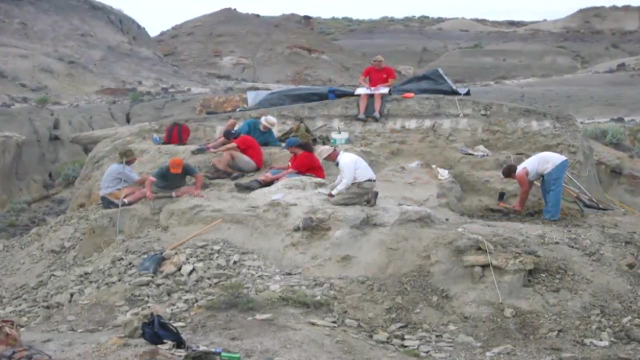 There's various other kinds of technologies that assist us in the field actually locating and positioning the fossil finds, because it's very important to us to know where in the rock column the fossil is found and also, of course, the geographic position of the fossil. 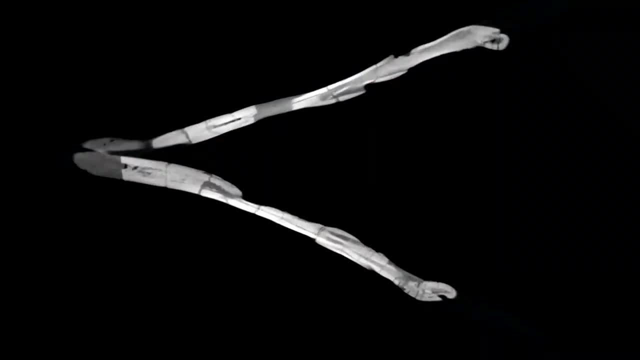 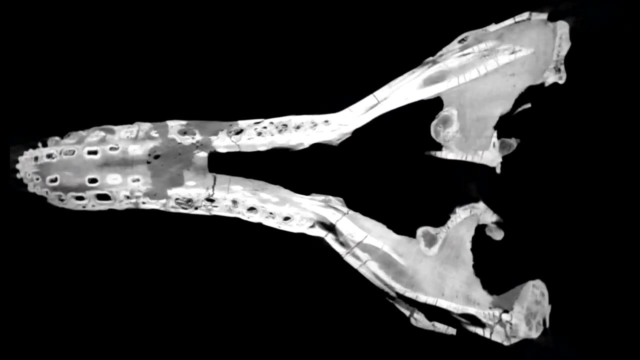 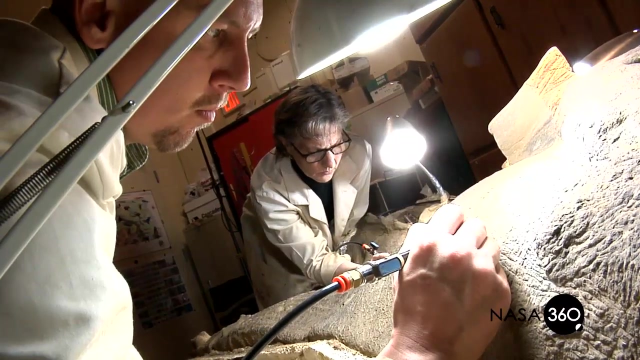 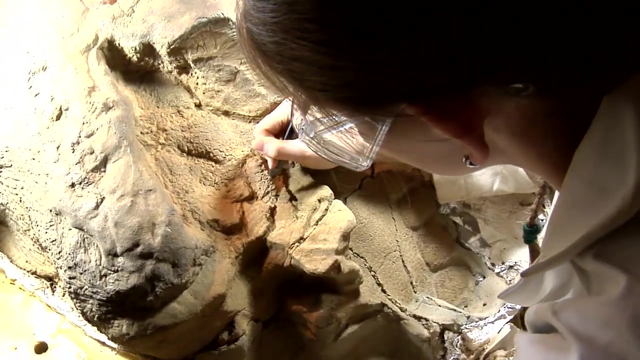 We also use CAT scans for determining the bone structures of skulls and also the size of brain cases in skulls- fossil skulls that have been found. So yeah, Technology is used extensively now in paleontology. We're preparing this for exhibit. The tail and one of the arms will be prepared and put on exhibit here at the North Dakota. 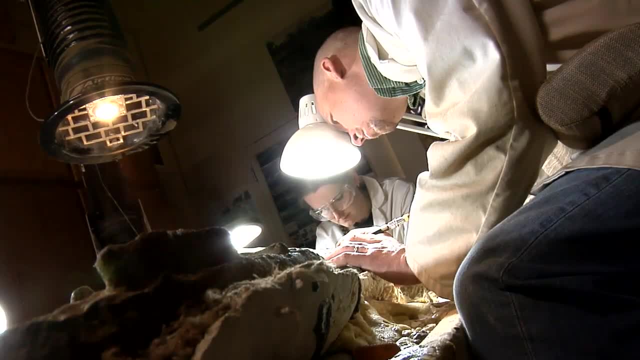 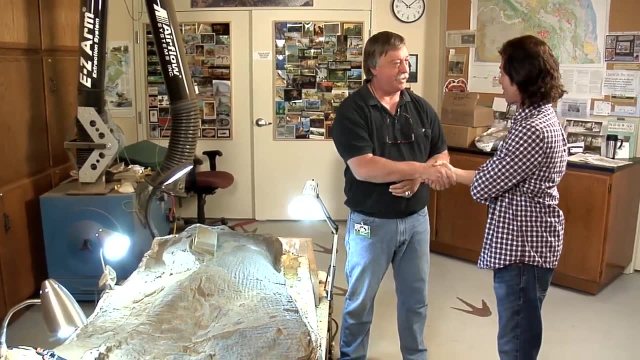 Heritage Center which is open to the public. So we plan to have it here for quite some time if people are interested in coming and seeing it. Good, Absolutely Well, Doctor. thank you so much for having us here at the North Dakota Heritage Center. 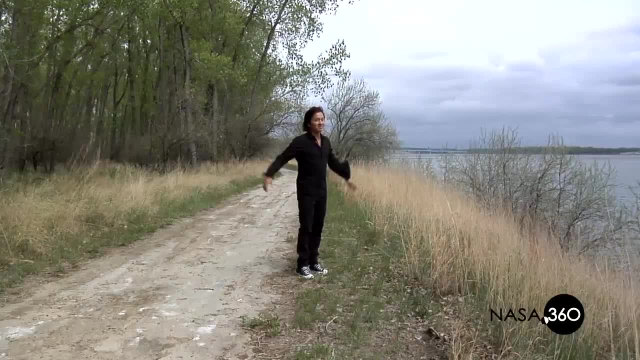 Sure, It's really good to have you here, Most definitely. Thank you, Hey. In a little bit I'm going to tell you how NASA is bringing history to life on the North Dakota Trail. So don't go anywhere, It's coming right up. 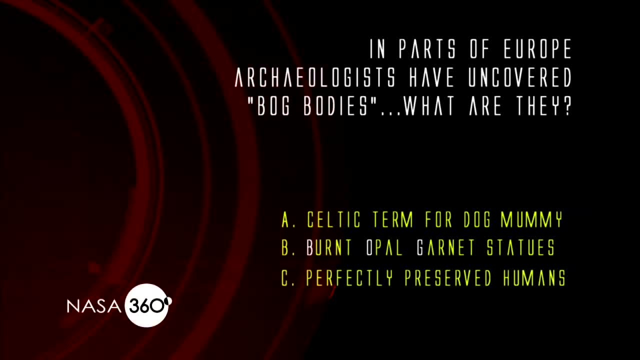 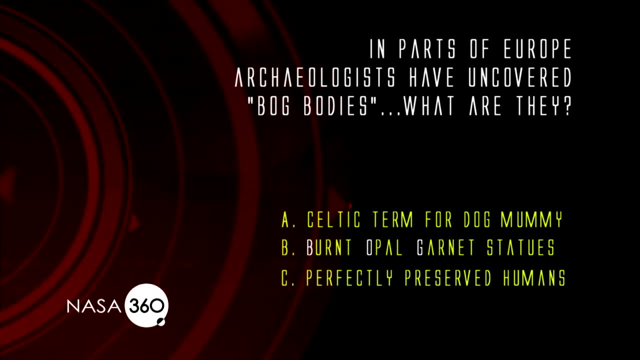 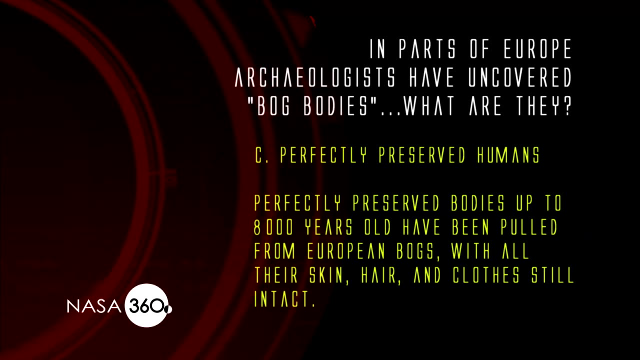 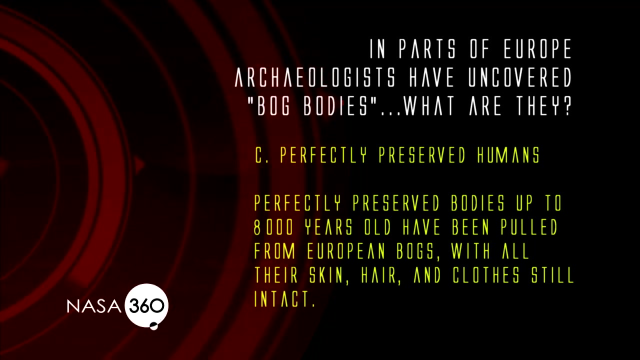 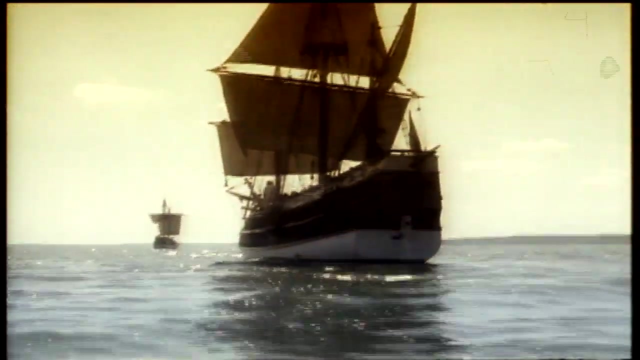 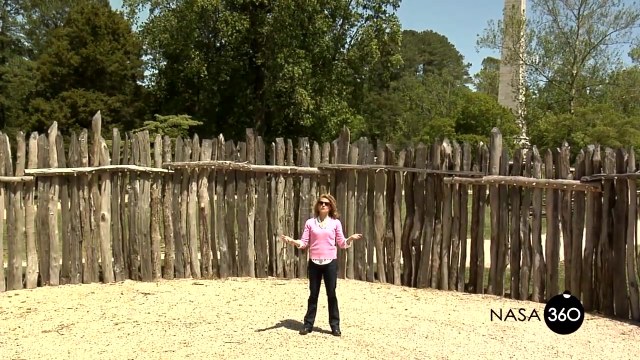 You're watching NASA 360.. Okay, So the first English settlers landed here in Jamestown in 1607, but the first years, oh, they were rough. In fact, for many years there was question as to whether this small fort would actually. survive. There was starvation and a lot of sickness, But thanks to some local Indians and some resupply from England, this small little fort held on and it began to flourish. In fact, from 1612 to 1698, Jamestown was the capital of the United States. Wow, Jamestown was the capital of the whole country. That changed when a fire swept through the statehouse and it forced the capital to be moved to Williamsburg. Just a few years later, Jamestown was gone, both physically and in memory. 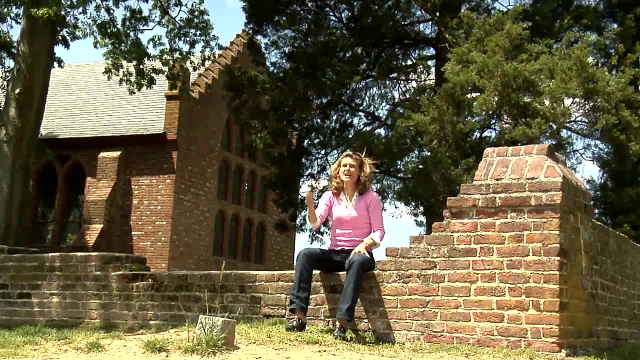 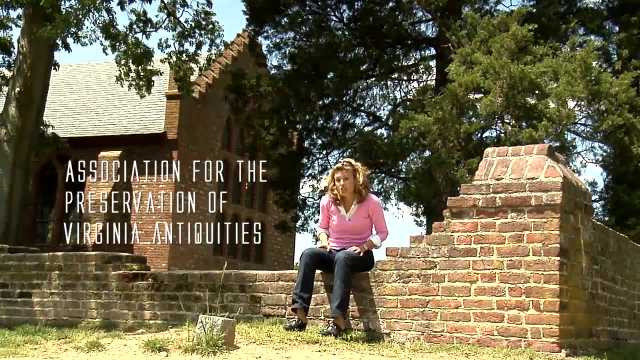 Over the centuries, people believed that the old fort and all of its artifacts had actually washed away into the James River. But that all changed in 1994 when the Association for the Preservation of Virginia Antiquities, or for short the APVA, commissioned an archeological dig. 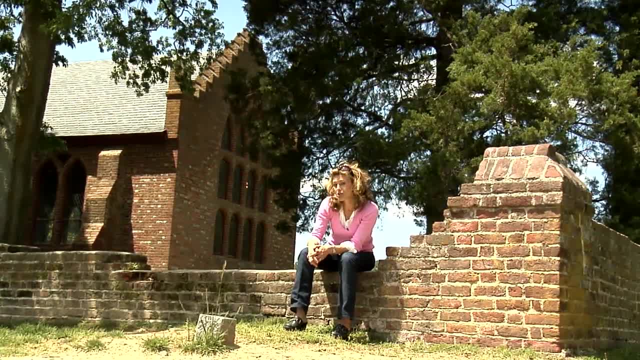 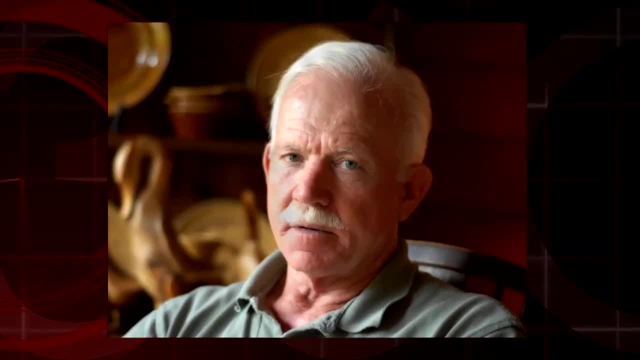 Wow, An archeological dig in the area where the original fort was thought to be. Why, Well, APVA lead archeologist Dr Bill Kelso believed the original fort had not been washed away at all. He had a hunch that he knew where to find the fort. 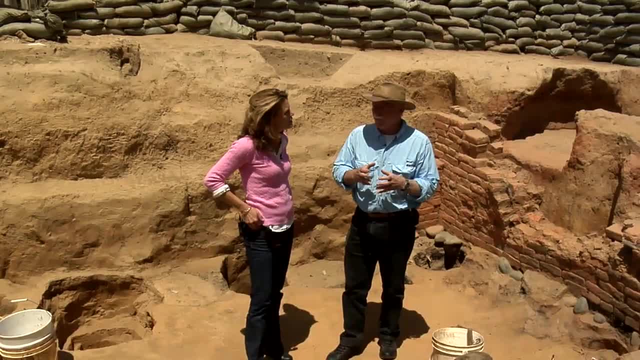 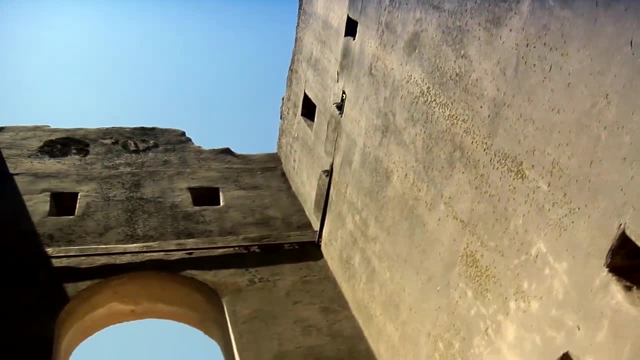 And this old church had something to do with it. Reason that I started digging where I did was that the church- there's a church tower here that's the only original above ground part of Jamestown 17th century and the church was originally in the area of James. 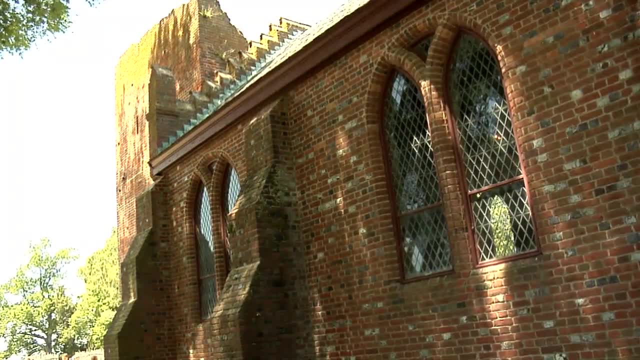 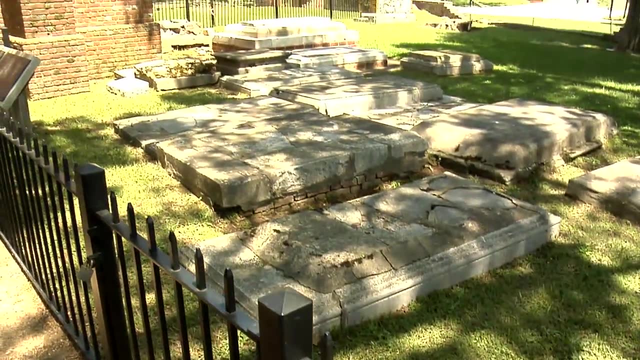 Wow, In the midst of the fort. One of the records said this: you know so well: it ought to be around here somewhere. so starting near the church was the key, and it was an area that had never really been looked at before. 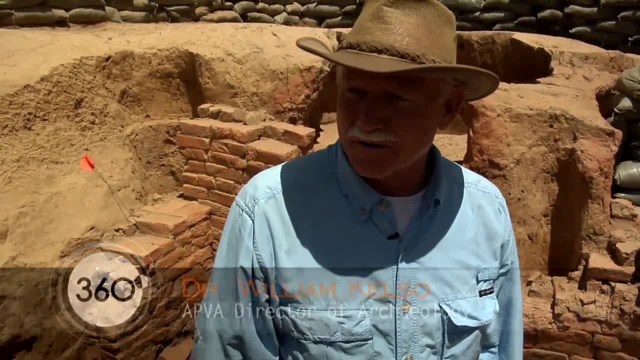 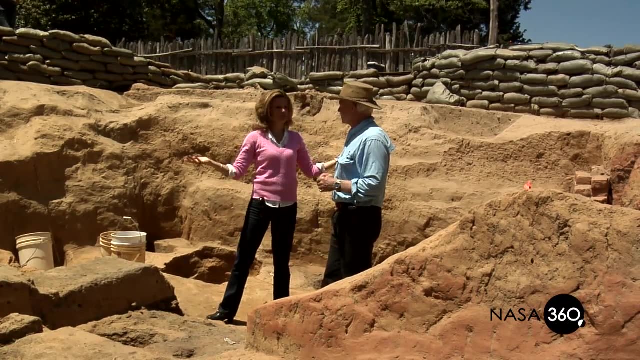 Ironically enough, it's high ground. it's really made sense. now that we know where the fort is, Can you walk me through the kind of the excavation process, the recording? we were talking a little bit about the technology and then where do the artifacts go from there? 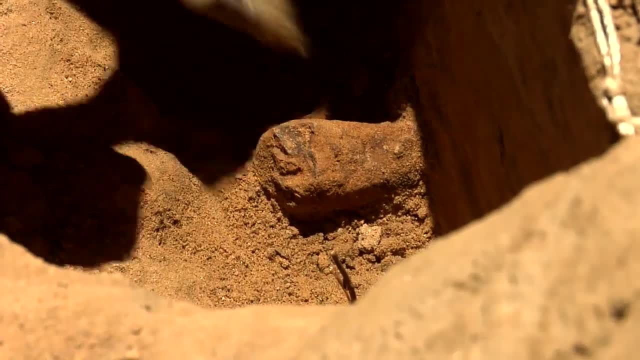 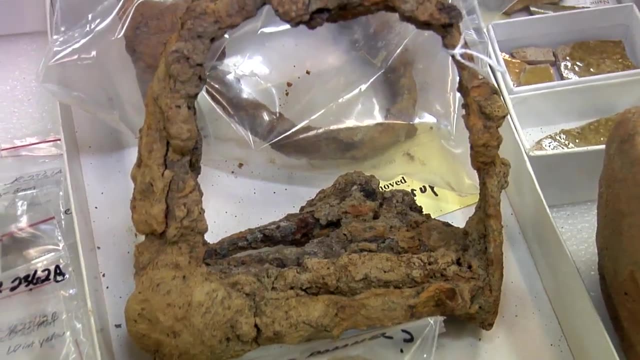 Well, artifacts are removed from their soil and once we understand the context, we call it where they're found: They're taken to a lab And they're washed, and then some of these, like these iron objects, would have to be conserved. 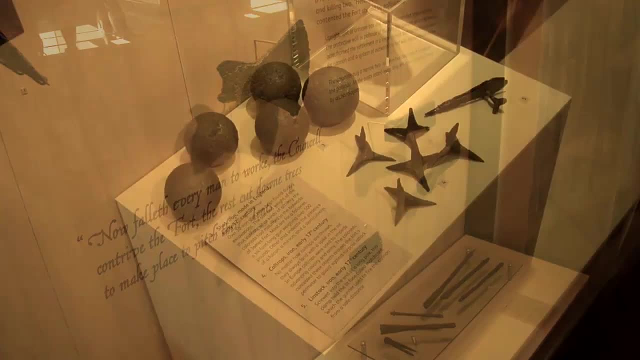 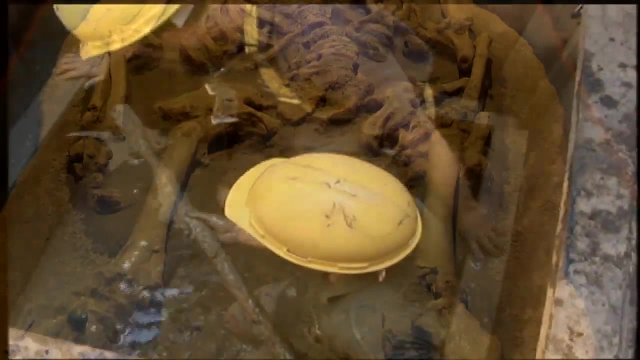 Some things- probably one or two percent of what we have here- will go on exhibit. We have a- you know- a museum here and there are other traveling exhibits and other things that we do just to tell the Jamestown story. How are we going to do this? 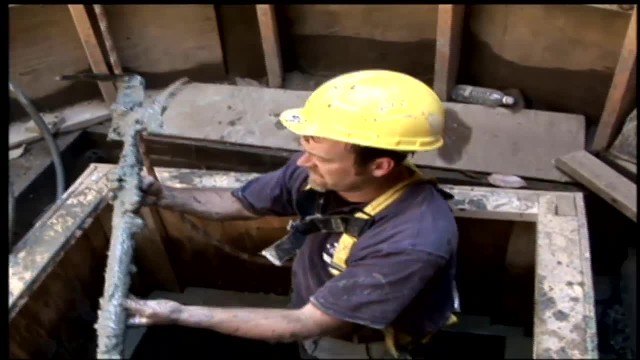 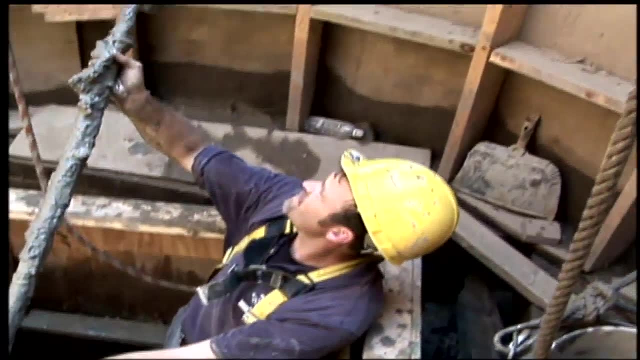 Oh my look at that. Oh my God, It's all metal down here. that's why it's locked together. That's Lord Delaware's That comes over to Lord Delaware. Dr Kelso, how long have you been an archaeologist? 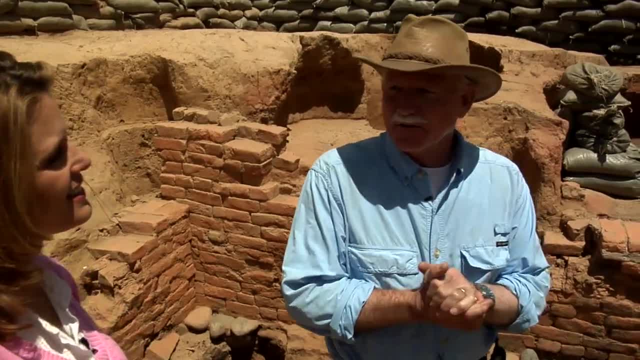 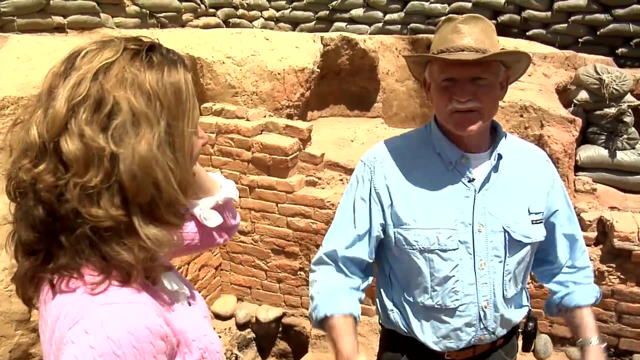 Well, I started probably 1607, something like that. Wow, you look great. Thank you very much. You're over 400 years old, gosh. It's been a while- 45 years, I guess I would say. 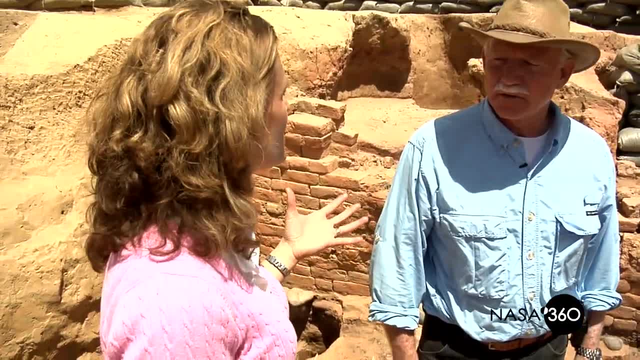 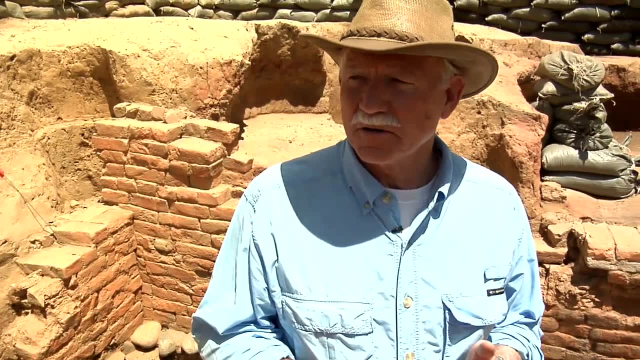 All right. so in that time, in those 45 years, tell me, what have you seen? what changes have you seen? technology, technological advances in archaeology. Well, the major technological advance. You would think that we would have invented x-ray vision, you know, and we'd save a lot. 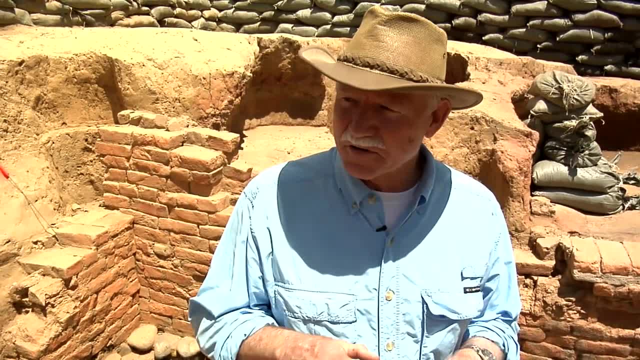 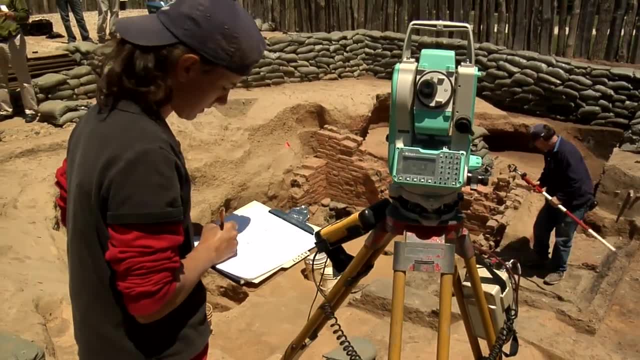 of digging Right, But that hasn't happened. There are certain machines that can give you some reading below ground without digging- remote sensing- But what I think the breakthrough has been has been in recording the record of archaeology, because archaeology, I think in the past, is something that's viewed as destructive. 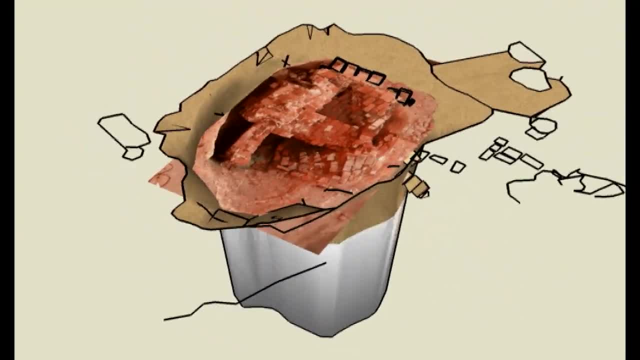 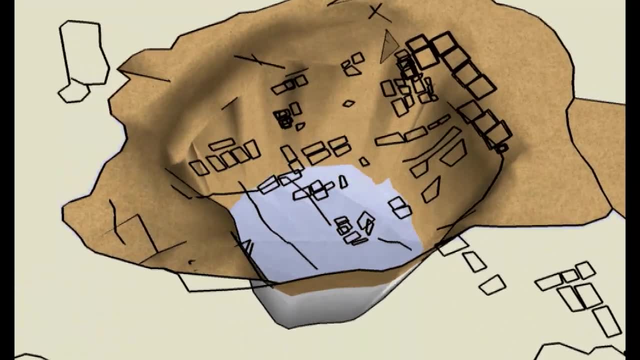 But now we have the technology through a GIS program that we can record almost in three dimensions. And we're close. If you can record in three dimensions then you can actually replicate the site again digitally and you know and re-look at it. 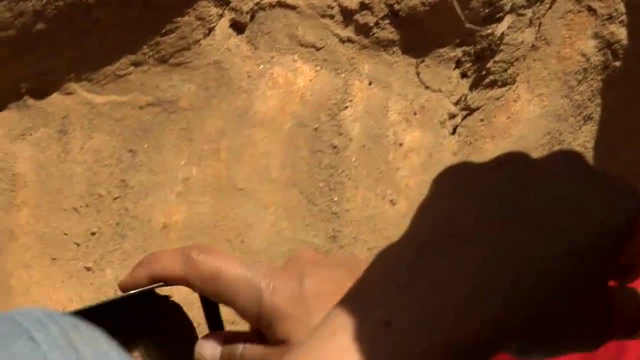 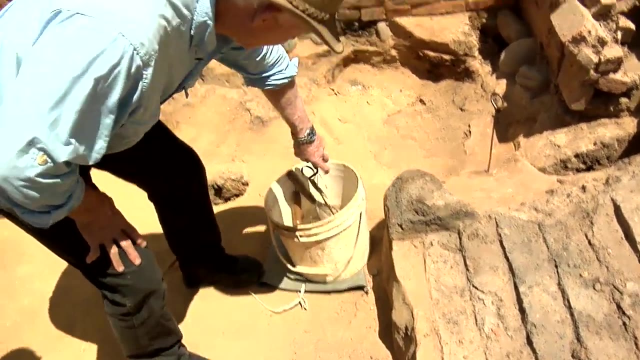 That still doesn't replace just, you know, blood, sweat and tears. I mean, it's just down, it's digging, it's stooping, it's using our main instrument here. It's just this small shovel and you know it takes a long time to dig out a hole like. 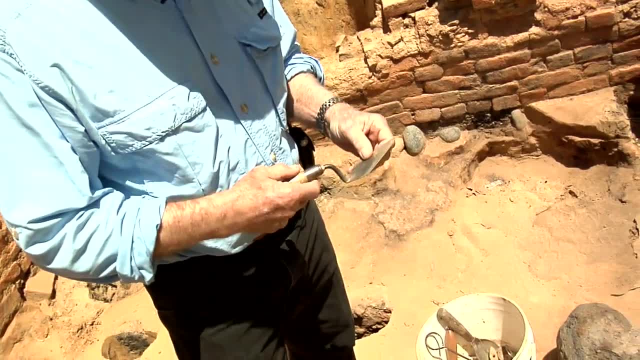 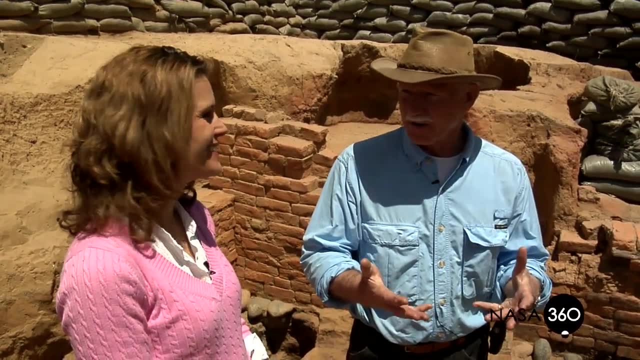 this with something like this, But we have to do that so that we don't disturb artifacts. So tell me about some of the amazing things you've found. Well, There are over a million artifacts in this project, But there are certain things that really do stand out. 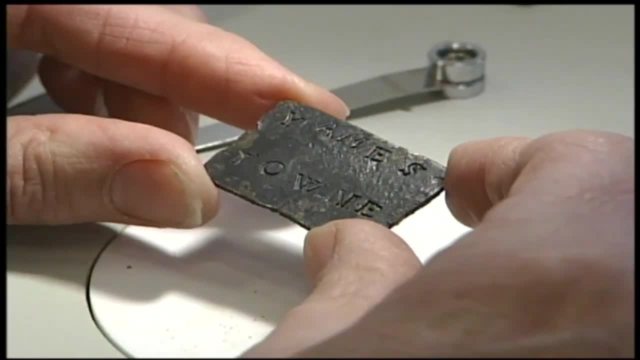 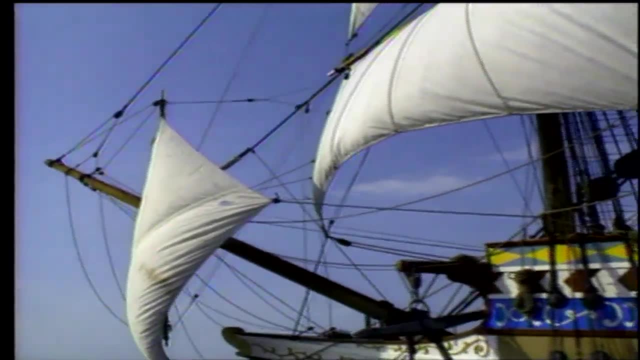 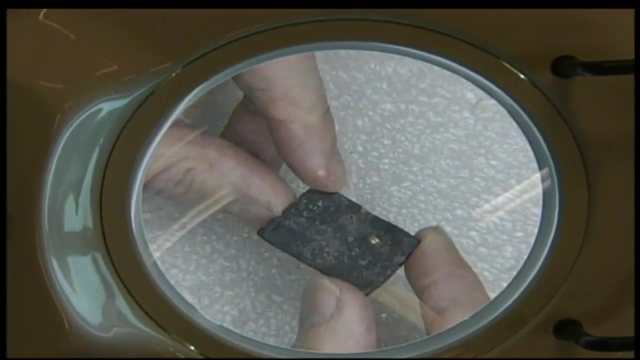 One of those things that stands out is a lead luggage tag with its destination stamped on it: Jamestown. This tag made the long journey from England to the New World on a wooden ship, then was discarded into the bottom of a well. After its rediscovery, 400 years later, it would again be making a long trip, this time. 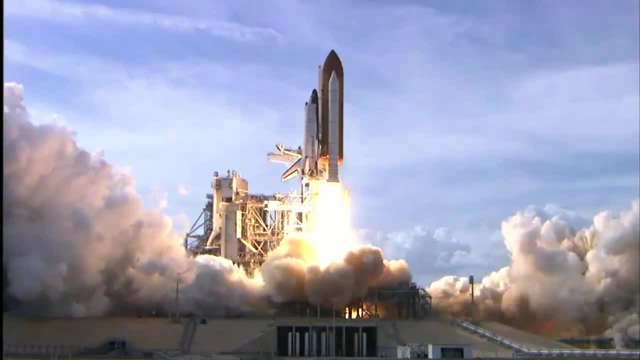 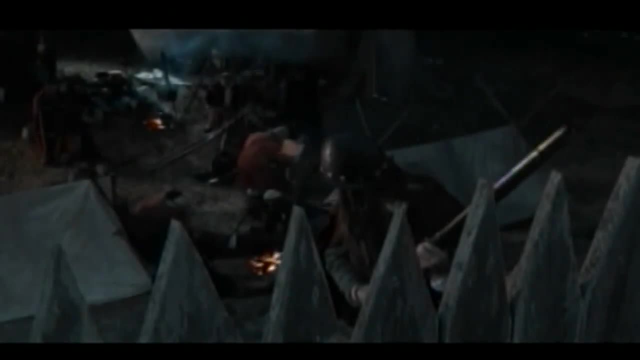 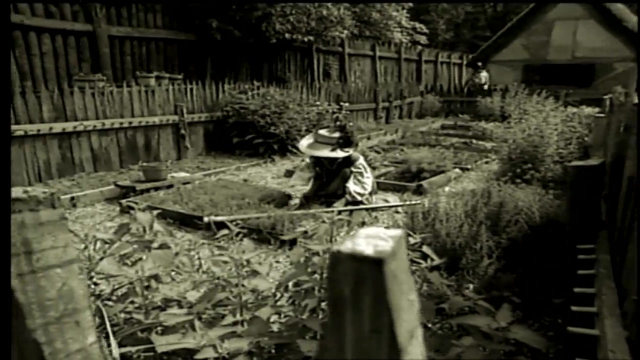 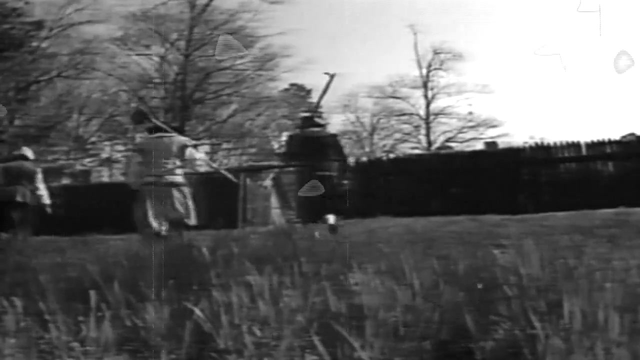 Virginia and and dress appropriately with armor and closed helmets, and because it was an alien environment, you had to put put some kind of a. it's almost like a. it is almost like a space station here or an outpost to begin to explore an unknown, and NASA's continuing to do that. right, and here's the colonization of the. 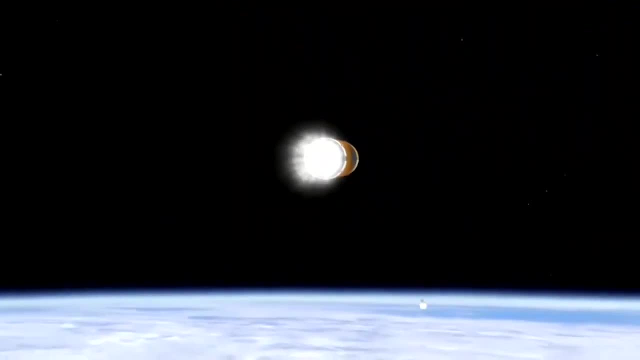 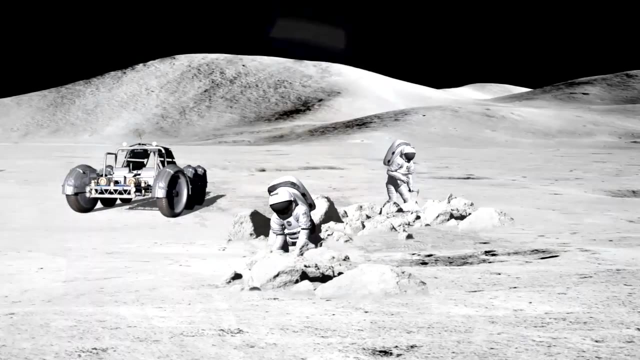 moon. and what are the problems? well, you got to get there, you got to, you got to have the right vehicles. what do you take with you? you know, how do you survive in this alien environment? you put in artificial surface around and you dress appropriately. so it is, it's really an age-old thing this whole psychological 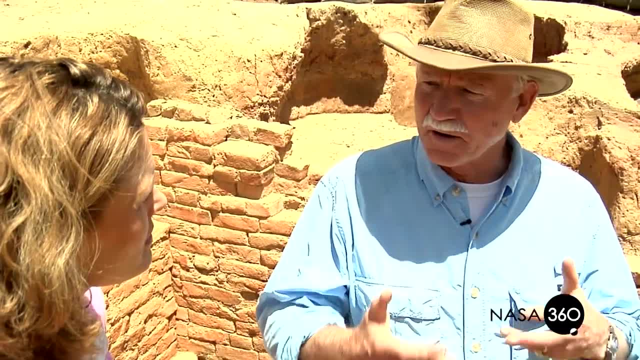 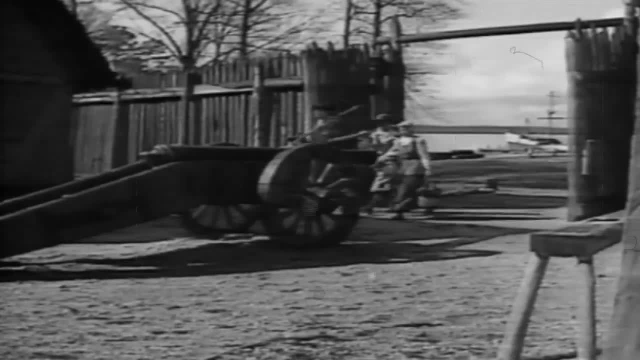 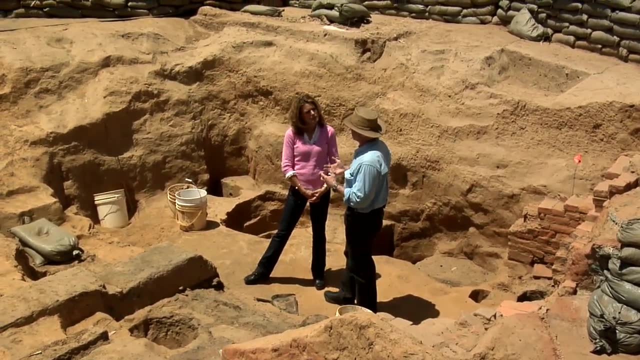 need to explore, a spiritual need to explore, I think, is still today, just as it was at the time of Jamestown. all right, so let's talk a little bit about this correlation between the early explorers- yourself, your Explorer- and then the future explorers. well, I'm kind of an explorer of explorers. there isn't. 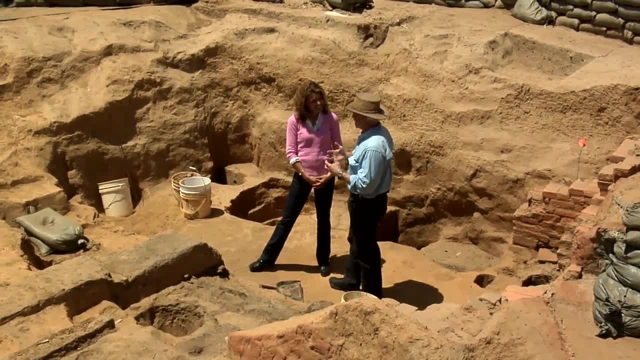 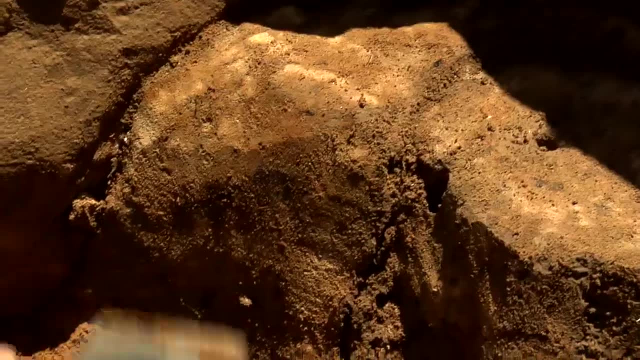 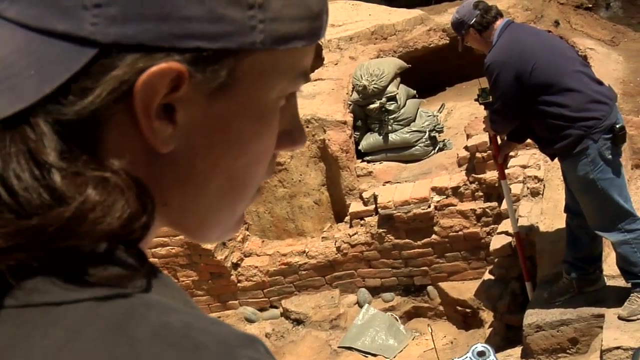 for us, I mean they, why we're trying to figure out what it was like to explore and discover, and we can. our projects called Jamestown rediscovery. you know, we're not discovering James, but we're rediscovering it, and a good example is this space here that here this was used as a laboratory to study the minerals. 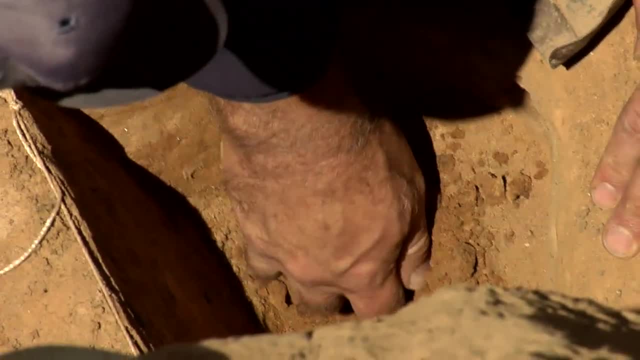 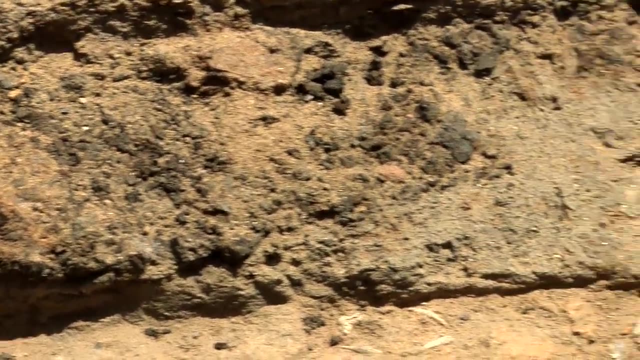 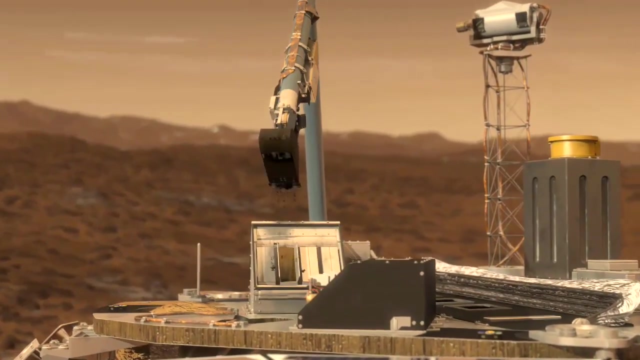 and the iron ore of this new land, see if it could be profitable right to come here, you know. so yeah, that's very similar to what I've read about explorations of in the world of thermodynamics. it seems to be interesting. yeah, in во, and they do drilling and they look at the materials and that's, that's what was. 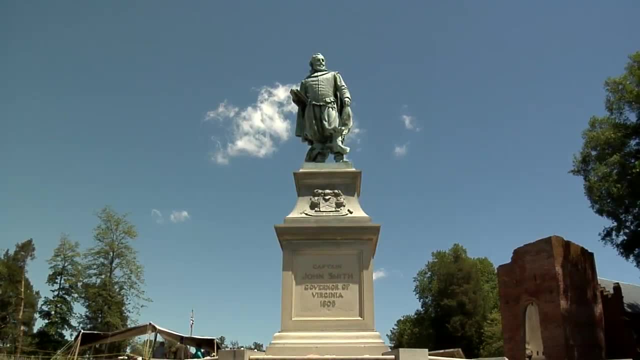 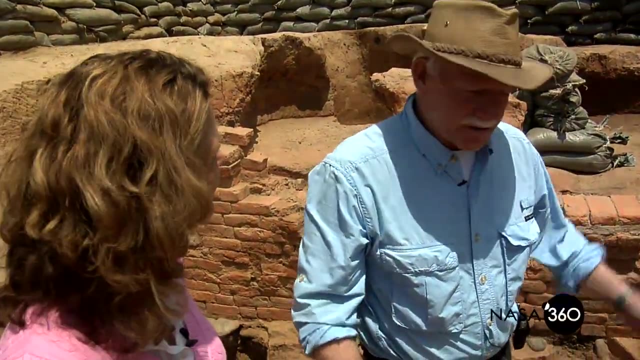 going on here, and so this space was where, I'm sure, people that you heard of before, John captain, John Smith, walk around. you know, maybe Pocahontas checking out the blacksmith shop that is so cool, that's, I mean, that's a mate, what? 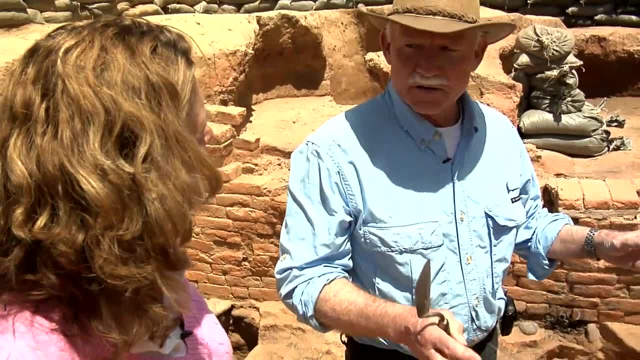 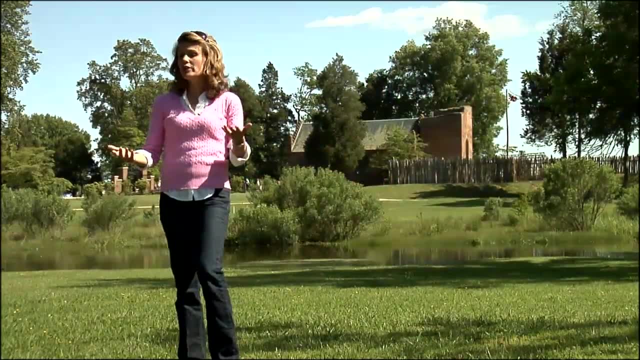 an amazing job you have. well, this- that's what that's the payoff is- is to tip to events happen. so then the events take on much more meaning than if you just read them in textbooks. Earlier, Dr Kelso mentioned the similarities between the 1607 Jamestown. 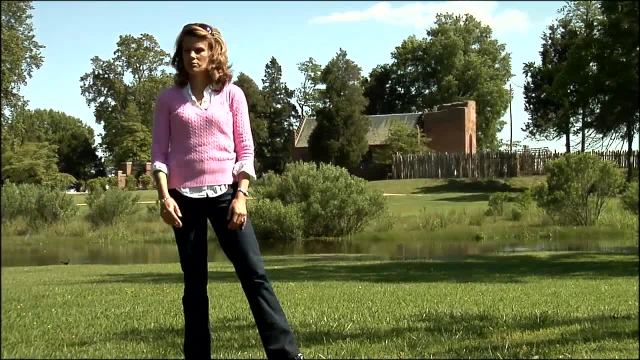 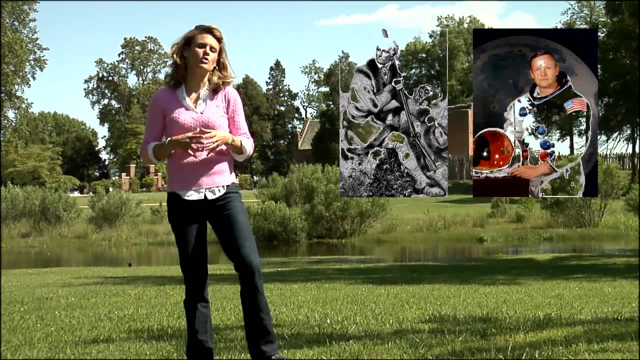 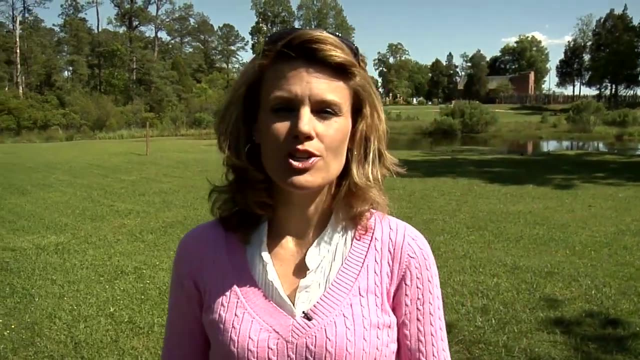 explorers and NASA's future space explorers. What about all the explorers in between? Guys like Daniel Boone, Neil Armstrong come to mind, as well as many countless others who have helped broaden our knowledge through exploration. Perhaps two of the most famous names in American exploration history are Lewis and Clark. 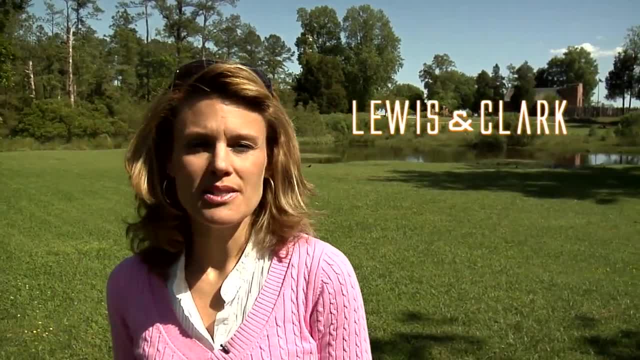 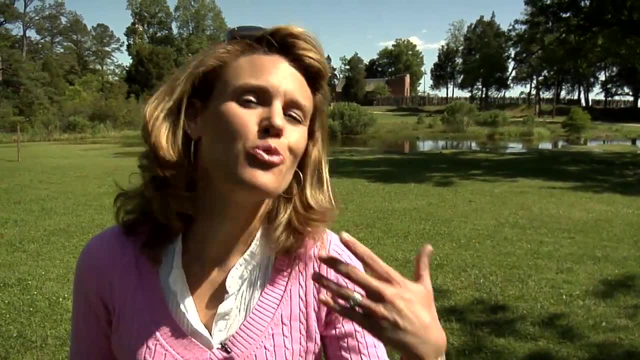 You ever heard of them? They blazed a trail through the American West, mapping out their path as they went. So what do you think? Did NASA have anything to do with the Lewis and Clark expedition? Well, not the original trip, but NASA is helping out now. 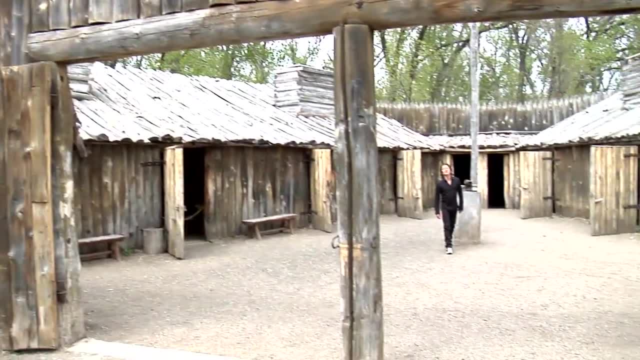 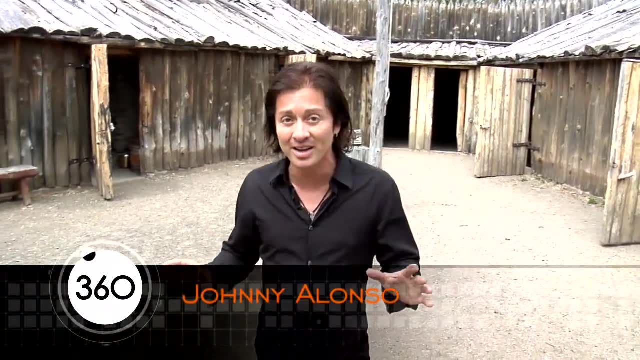 Johnny Alonzo will tell you all about it. All right, so we've seen a lot today how NASA's helping archeologists and paleontologists through remote sensing. These remote sensing devices have helped us unearth some really cool findings in places like Cambodia, Central America and the American Southwest. 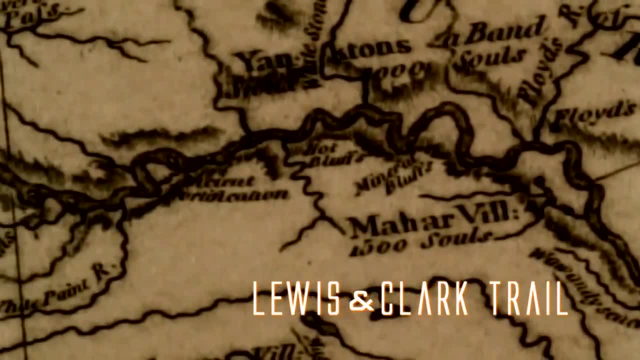 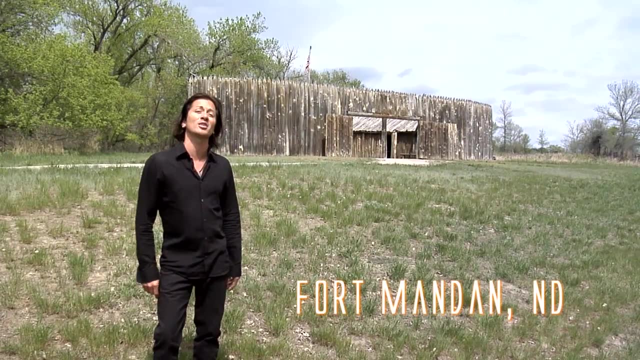 And they've also helped along one of the most famous trails in American history- Okay, The Lewis and Clark Trail. To find out how NASA helped map this 200-year-old trail, I rolled up to Fort Manda in North Dakota, to where Lewis and Clark spent their first winter. 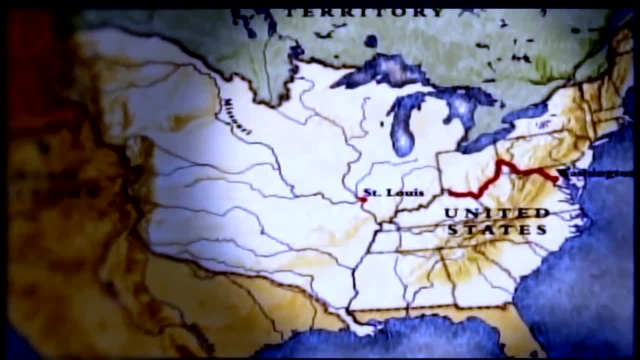 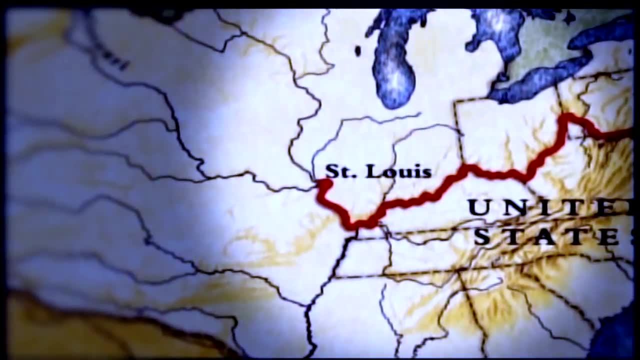 Before we get into NASA's involvement, let's go back a few hundred years to the beginning of the Lewis and Clark expedition. Back in 1804, when the expedition began, we knew almost nothing about what was to the west of St Louis. 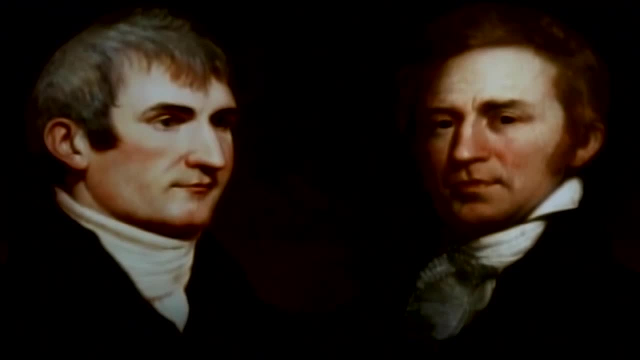 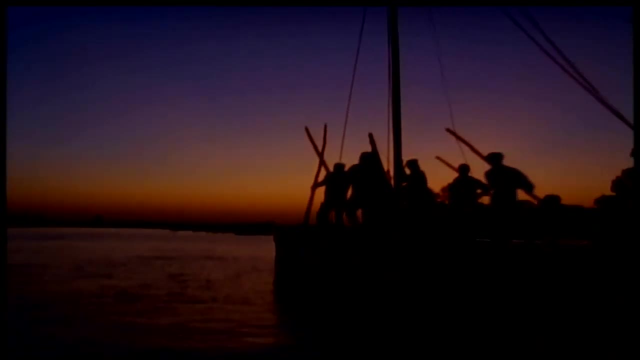 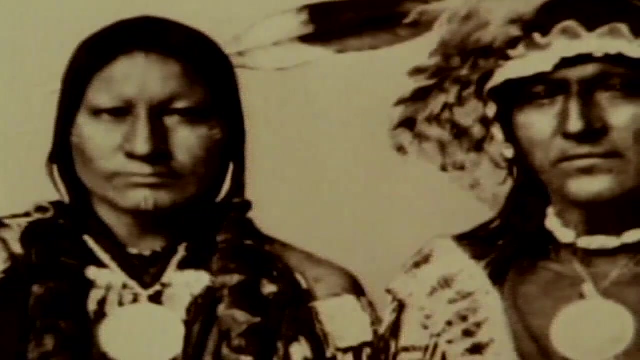 So President, Thomas Jefferson commissioned Meriwether Lewis and William Clark to lead an expedition west to find the first all-water route to the Pacific Ocean. This was an epic journey Taking several years and 3,700 miles to complete. During this trip they collected samples of plants and animals, met many of the different 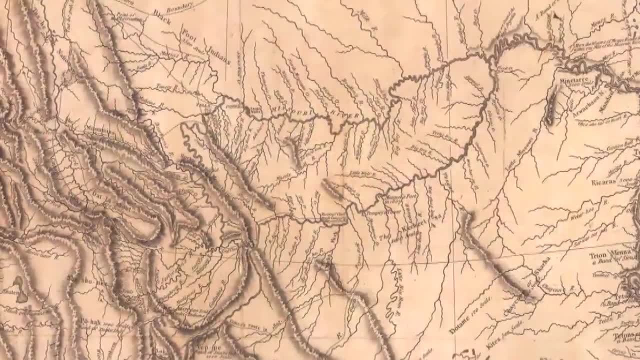 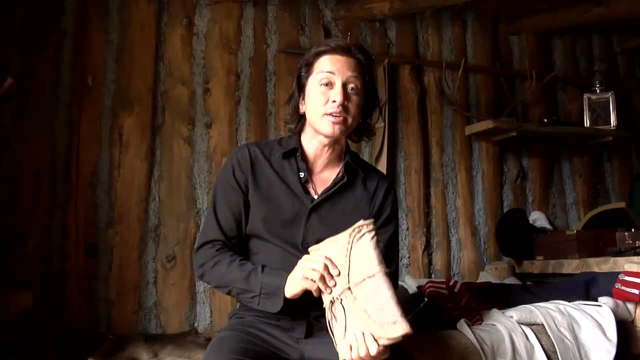 Indian tribes of the west and brought back detailed data about the route that they had taken. But even though they brought back some pretty good maps and data, they still weren't 100% accurate. That's because most of these journals weren't written right away or they were written after. 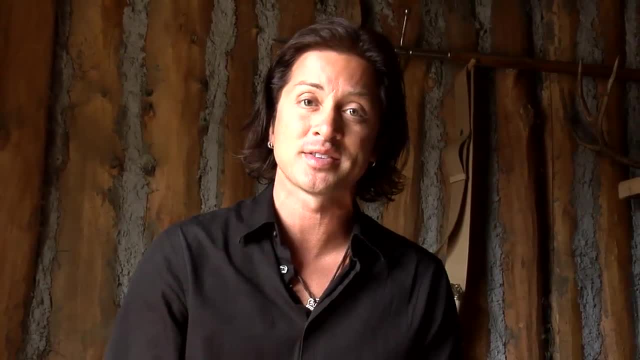 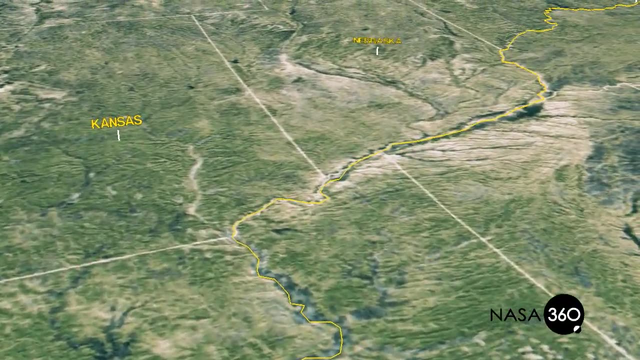 a hard day's travel, And many of the entries contained geographical inaccuracies. So this is where NASA comes in. Researchers from NASA's Stennis Space Center took the maps of Lewis and Clark, St Louis and Clark, and combined them with high-resolution images taken from satellites and aircraft. 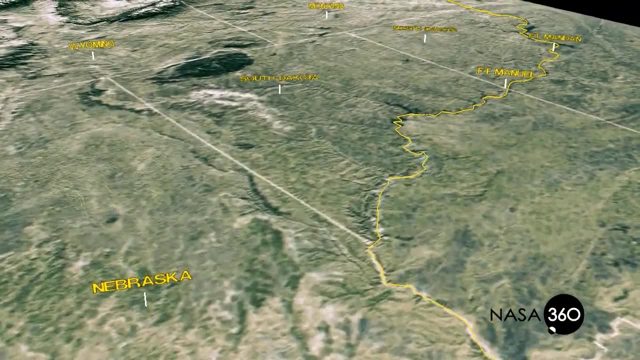 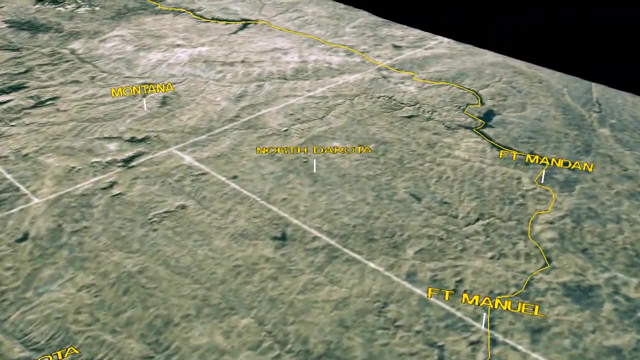 They created maps with a 360-degree view of an area where the explorers traveled. From that view, archaeologists could follow the trails as if they were flying over the actual landscape, in real time and in any direction or angle they chose. 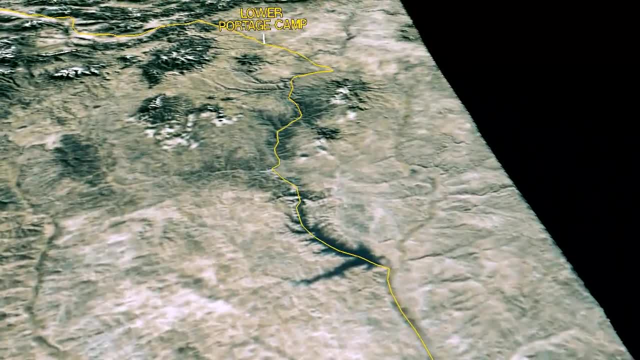 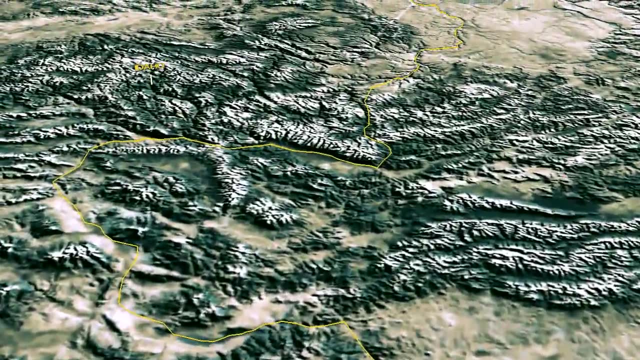 Researchers pored over these maps, looking for telltale signs of human disturbances unique to the Lewis and Clark expedition. With this technique, archaeologists were able to narrow down some of the possible sites from many miles to a few inches. This information is helping to find Lewis and Clark artifacts that provide a clearer 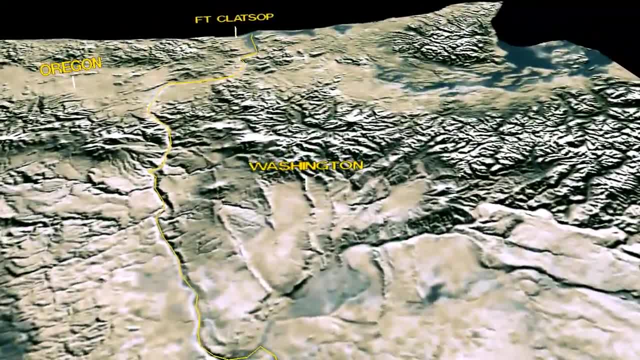 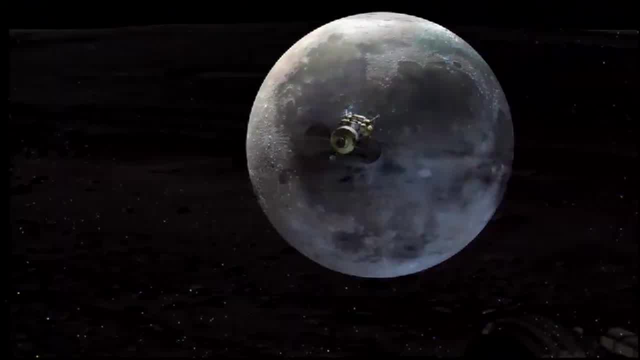 understanding of the expedition and what the lives of those early explorers had been like. And don't forget, NASA has a new generation of explorers too that will soon be going back to the Moon and on to Mars. So in the future, when we talk about great explorers, there's no doubt that NASA's 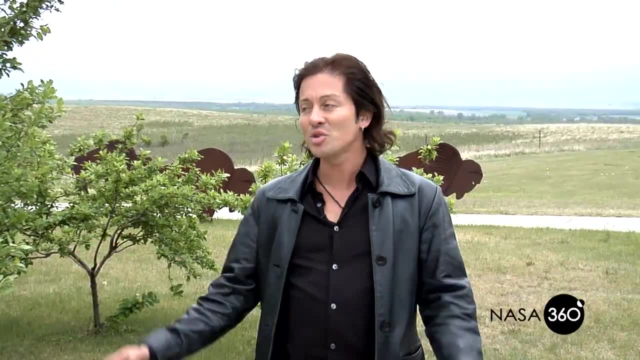 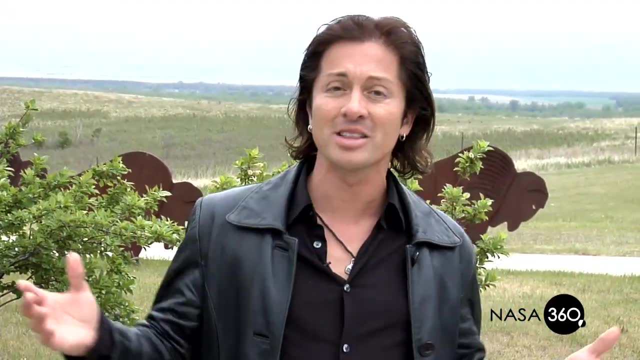 astronauts will be on the list. It's amazing, isn't it? Just when you thought you knew everything about NASA, we throw something else at you. So, as you can see, NASA is not only trying to help shape our future, it's also making